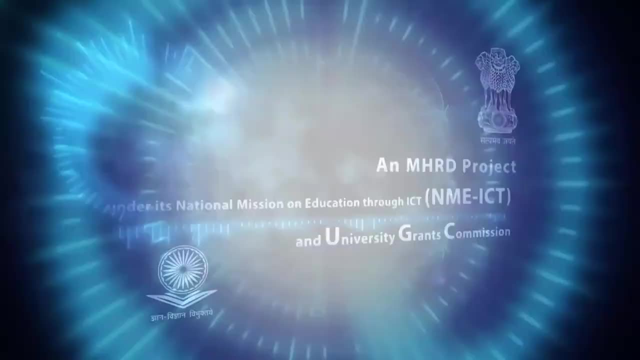 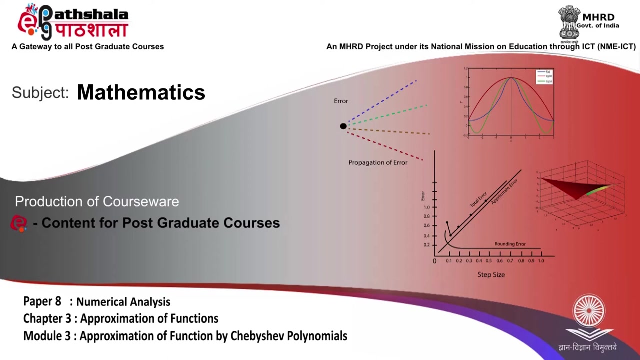 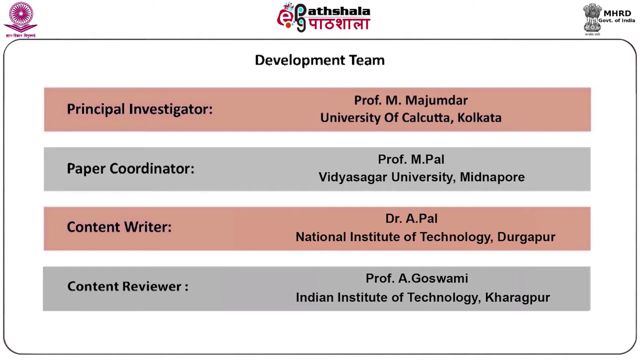 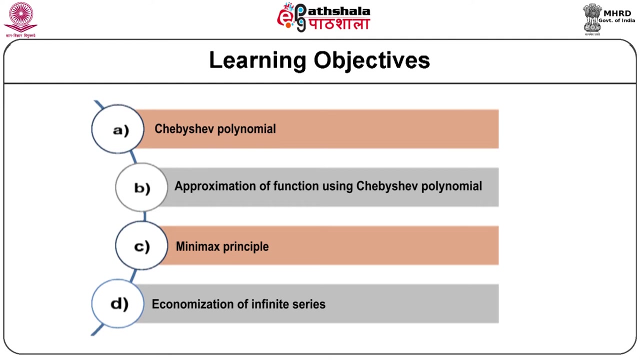 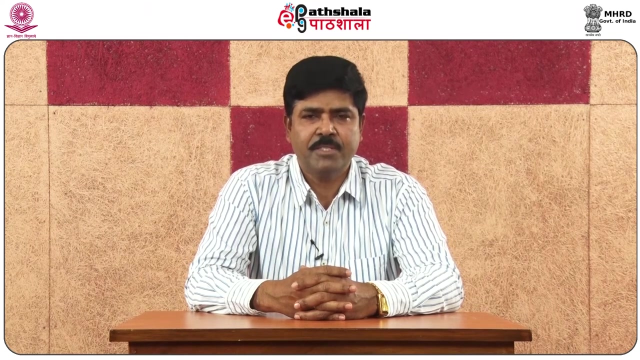 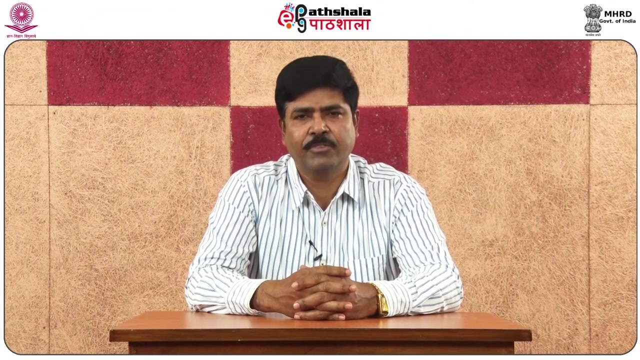 Thank you for watching. This is last and third module of chapter 3.. In module 2 of this chapter, we have described some methods to approximate a function to a polynomial or to another function using orthogonal polynomials or without using orthogonal polynomials. 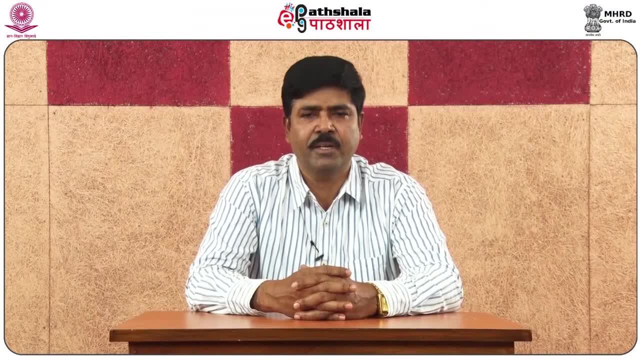 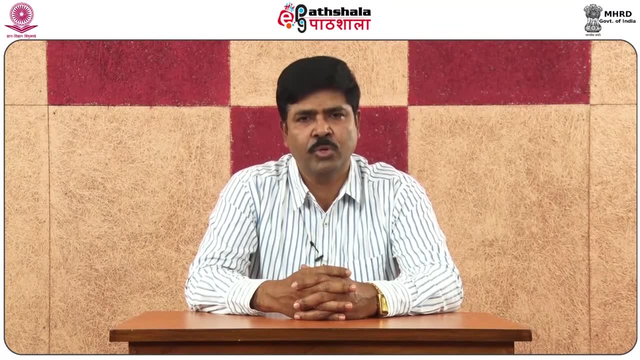 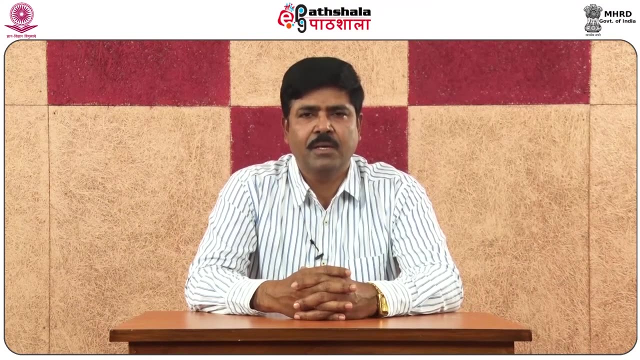 And we have shown that use of orthogonal polynomials reduces the computational efforts. In this module we shall consider CBC polynomials to approximate a function to a polynomial And we shall show that these orthogonal polynomials are efficient compared to other polynomials In this module. 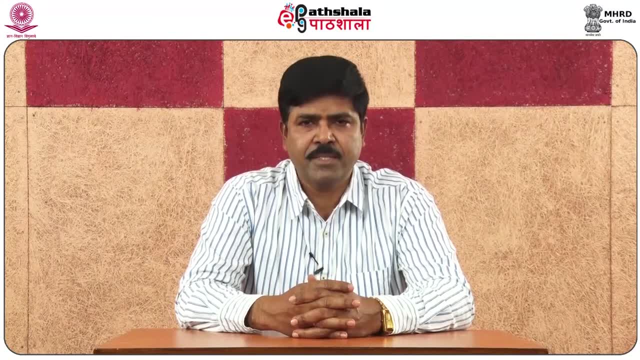 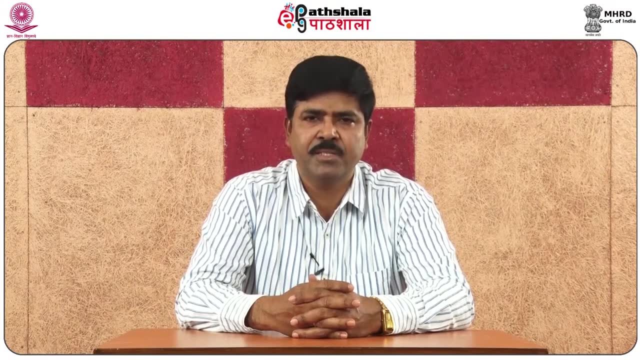 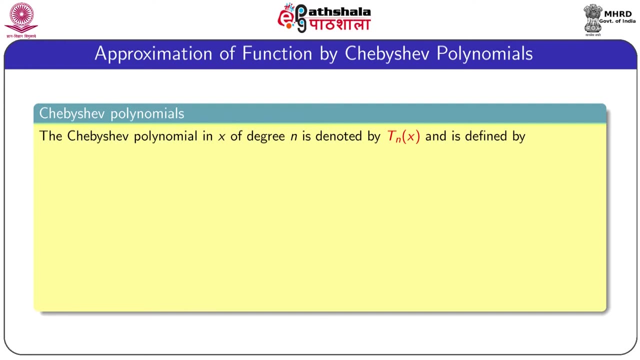 we shall show that any function can be expressed in terms of CBC polynomials. if the function can be expanded or not, Let us see how to formulate the polynomial. Let us try toidade with the help of the Taylor series method. First, we define CBC polynomial. The CBC polynomial is denoted by Tn, x, where n represents 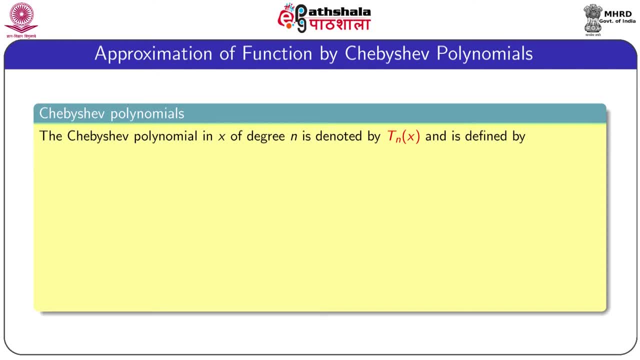 the degree of the polynomial and x is the variable and which is defined by Tn of x equal to cos of n into cos inverse x, And this is defined on the interval, close interval minus 1, 1.. And n is valid for n into cos inverse x And there also theBut the polynomial. denotes the degree of the polynomial. So if we take the polynomial and we find ta n of x, the way it is calculated, for x is equal to cos of n into cos inverse x. Now we can also write the interval minus 1, 1.. This is what we can do. This is the expression of the polynomial. 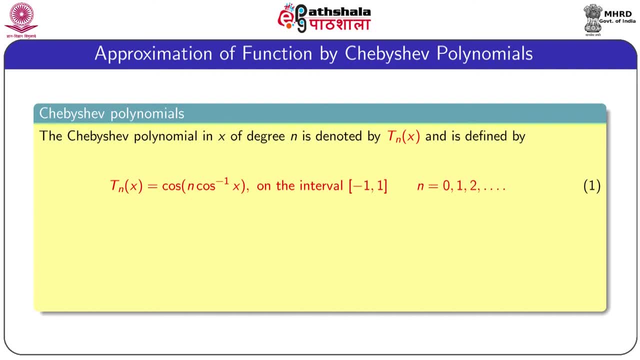 for 0,, 1,, 2 and so on. This polynomial can also be written as: Tn of x equal to cos n theta, where x equal to cos theta. These polynomials look like a trigonometric function, but this is an algebraic function by expanding the cosine function and cos inverse function. 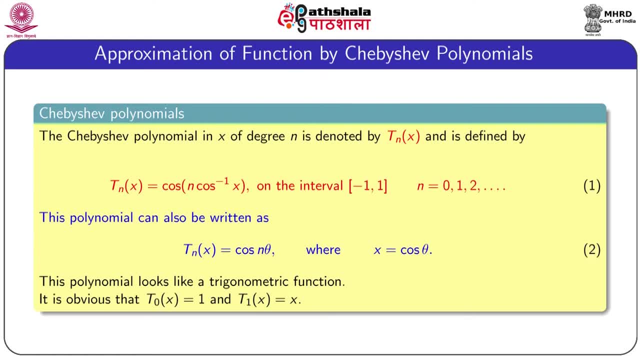 And particularly when n equal to 0, T0x equal to 1 and T1x equal to x. This is the initial values of the polynomial Tn for n equal to 0 and 1.. We know that the function cos theta. 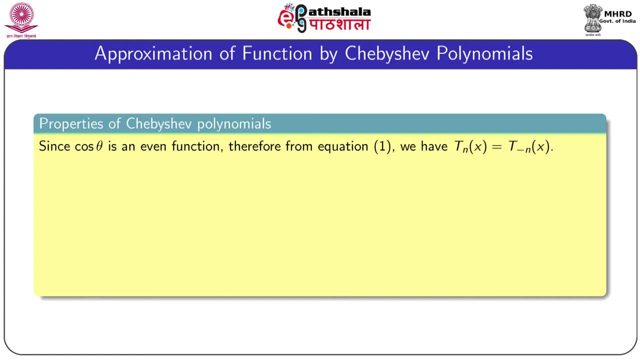 is an event function. Therefore, from equation 1, that means from the definition of Tn, we can show that Tn equal to T of minus n of x. Also, it is easy to verify that T of 2n of x equal to T subscript twice n of minus x. 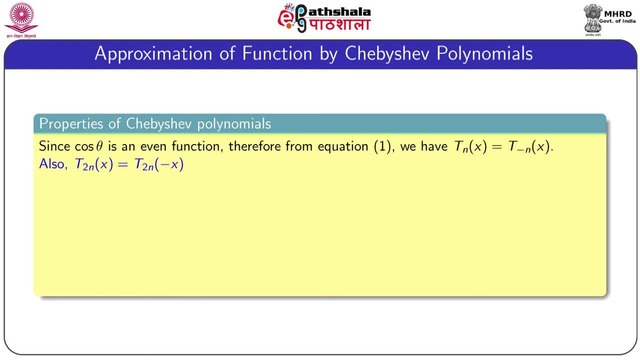 That means the Szebeski polynomial is, even when the subscript is even, And also T, subscript 2n plus 1 of minus x equal to minus of T of subscript 2n plus 1 of x. This shows that the Szebeski polynomial is an odd function if the degree of the polynomial is odd. 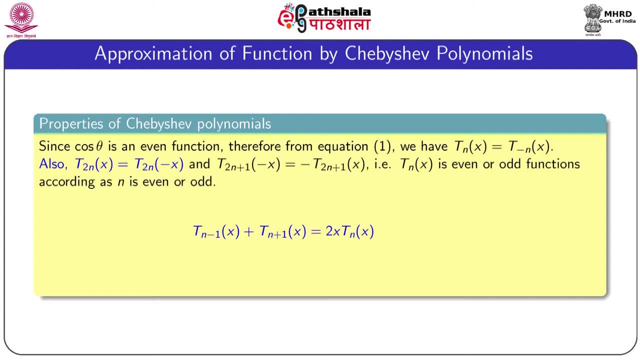 Also, we can prove that T of x plus T of x equal to twice x into 2Tnx, That is, T n plus 1 of x equal to twice x into 2Tnx. This is true for all n equal to 1,, 2,, 3 and so on. This is the recurrence relation for 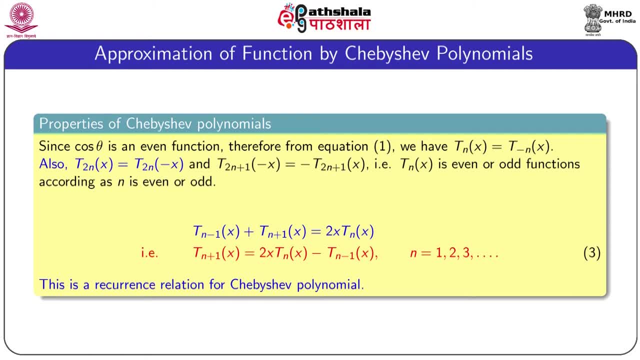 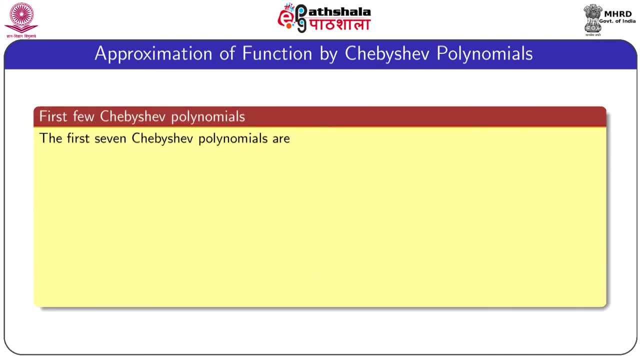 Szebeski polynomial. So from this recurrence relation we can generate all order Szebeski polynomials starting from n equal to 1.. So from this recurrence relation we can generate any order Szebeski polynomial. So first 5, first 7 Szebeski polynomials. 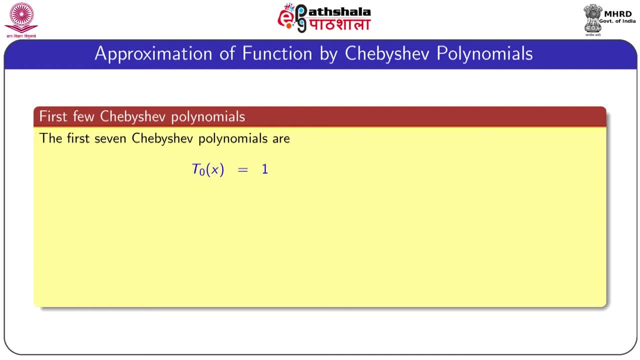 are: T 0 x equal to 1,. I have mentioned already this particular polynomial: T 1 x equal to x. T 2 x equal to twice x square minus 1,. T 3 x equal to 4 x cube minus 3 x. T 4 x equal. 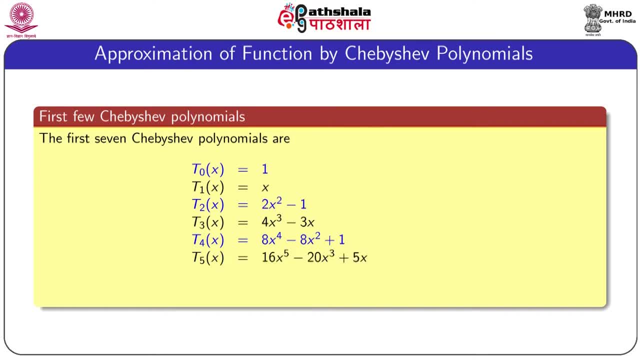 to 8 x, to the power 4 minus 8 x, square plus 1.. This one: T 5 x, T 6 x, T 7 x. Note that the function say T 3 x, T 5 x, T 8 x plus 1, they are the 1. And the function is that. 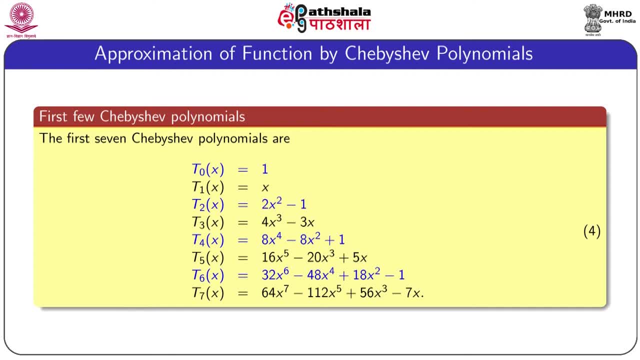 t7x are odd functions and each power of each term is odd. And in the function t3x the power of x is 3 and 1.. Similarly, in the function t5x the power of x are 5,, 3,, 1.. That means 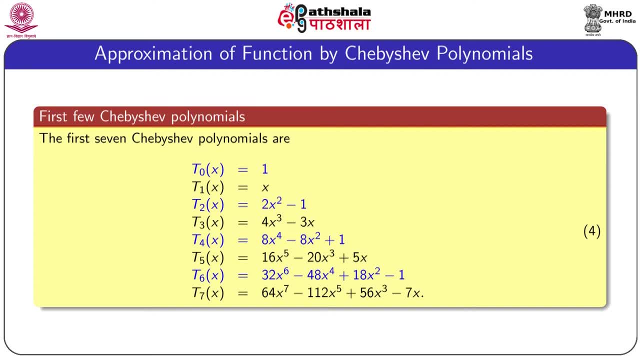 all the power of x are odd. Similarly, the powers of x in t7x are 7,, 5,, 3 and 1.. That means all the powers are odd. for odd suffix polynomials And for even suffix polynomial the power of x are even. For example, in t6, the power of x are 6,, 4,, 2 and so on. 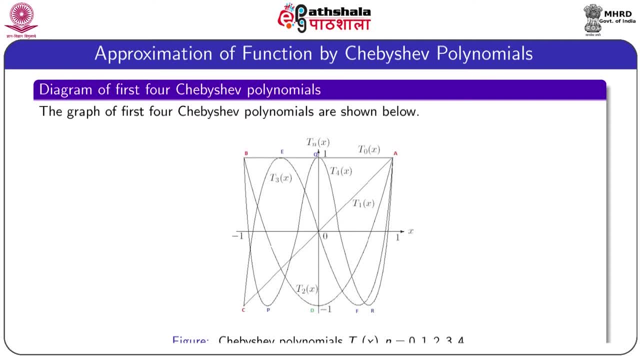 So these are the graph of first four C-Base wave polynomials. The first graph is AB, the line AB. This one represents the polynomial t0x. The second polynomial t1x represents is the line that is aoc and the polynomial t2x is the curve bd, The polynomial. 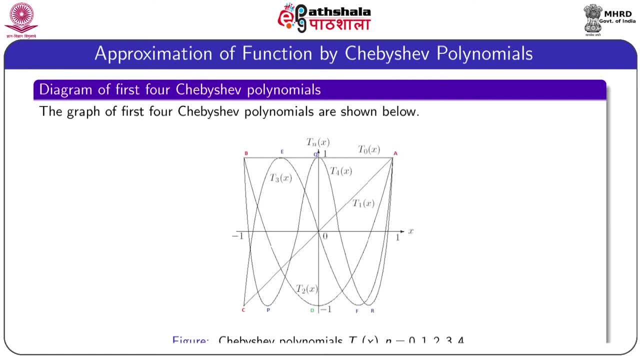 t3x is e and f. the polynomial t4x is b, then p, then q, then and a. So these are the first 5, including the strutting polynomial, the firstbrand polynomial. Next, we have ability bound this line to those where we are writing A, b, p and c, So we 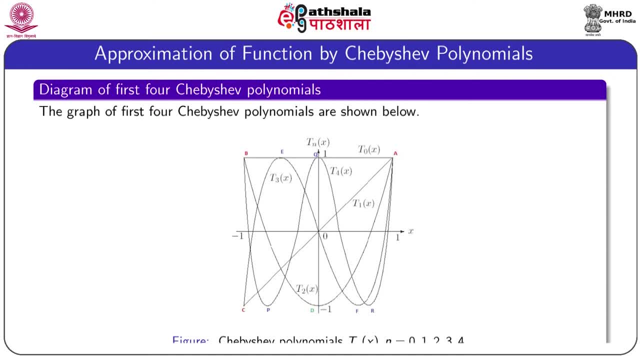 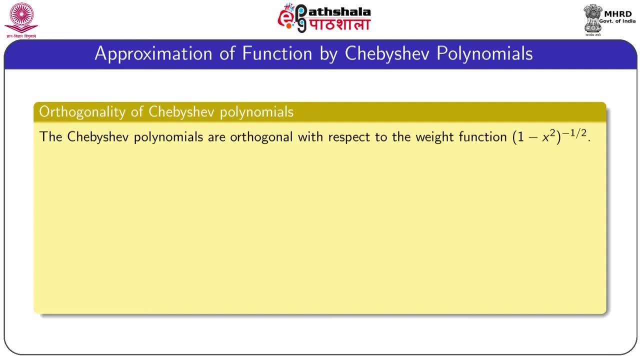 the phi polynomial or Sibeshi polynomials. It is interesting that the Sibeshi polynomials are orthogonal, with respect to the weight function, 1 minus x square whole, to the power minus half, So Wx equal to 1 minus x square power minus half. So to prove the Sibeshi 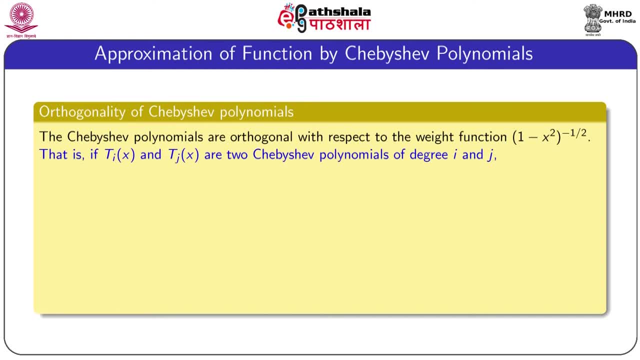 polynomials: orthogonality of Sibeshi polynomial. we consider two Sibeshi polynomials of degree i and j, and these are denoted by Tix and Tjx. If the polynomial Tix and Tjx are orthogonal, 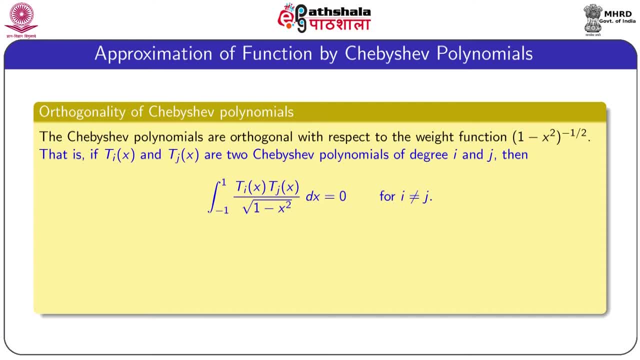 with respect to the weight function, 1 minus x square power minus half, we have to prove integration minus 1 to 1 Tix into Tjx whole divided by root over 1 minus x square dx equal to 0 for different i and j. If i and j are equal, then the value of this integration 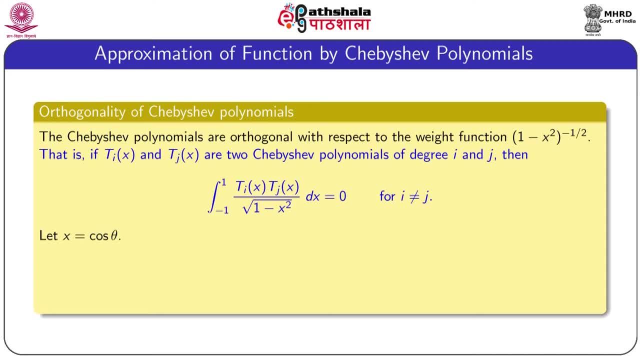 is non-zero. To prove this expression or to prove this result, we consider x equal to cos theta. Then the integral is denoted by i, where i equal to integration minus 1 to 1 Tix into Tjx whole divided by root over 1 minus x square dx equal to: after substitution: x equal to cos theta. 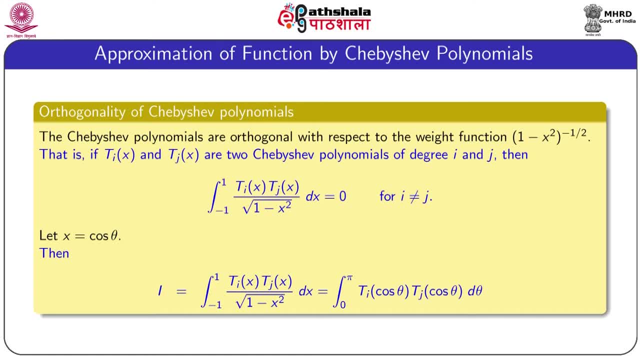 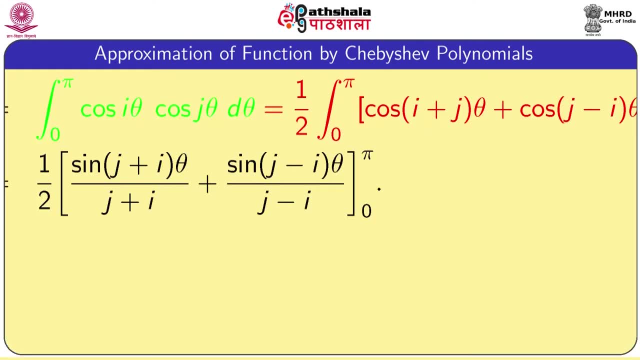 This integral becomes integration 0 to pi T i of cos theta into Tj of cos theta d theta. Thank you, That is i equal to integration 0 to pi cos i theta cos j theta d theta. equal to half of integration: 0 to pi cos of i plus j theta plus cos of j minus i theta d theta After. 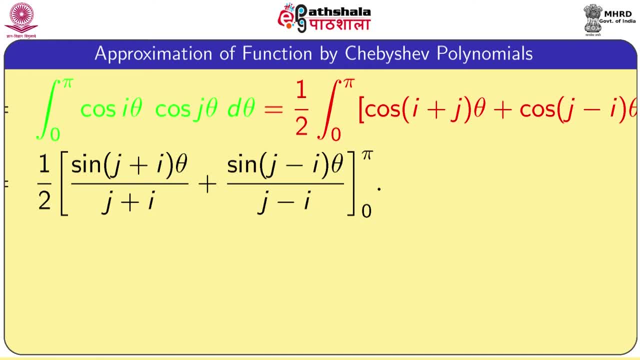 integration. it becomes half of sin j plus i, theta whole divided by j plus i, plus sin j minus i- theta divided by j minus i. Lower limit is 0, upper limit is pi. Now it is easy to observe that when j and i are different, then the value of this integration 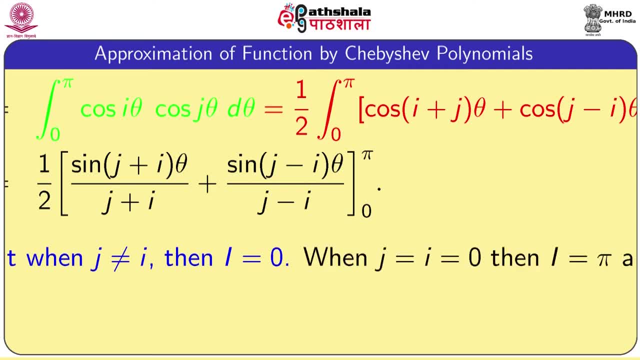 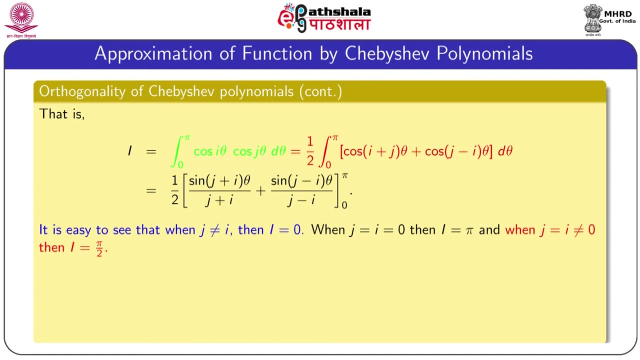 is 0. That means the value of i is 0. When j equal to i, equal to 0,, then from the green expression or green integral, we can easily shown that i equal to pi. And when j equal to i but not equal to 0,, then the value of the integration is pi by 2.. And this is obtained. 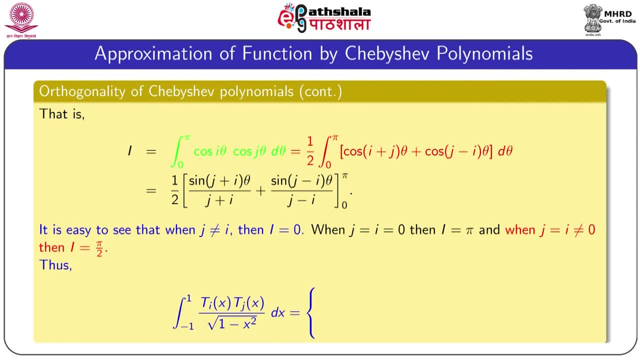 from the red mark: integration. Thus integration minus 1 to 1. t i x into t j x whole divided by root over 1 minus x square d x equal to 0. if i and j are different, equal to pi. if j equal to i, equal to 0 and it is equal to pi by 2. if j equal to i but not equal to. 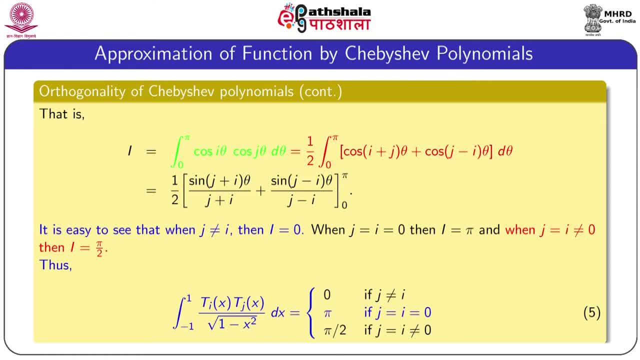 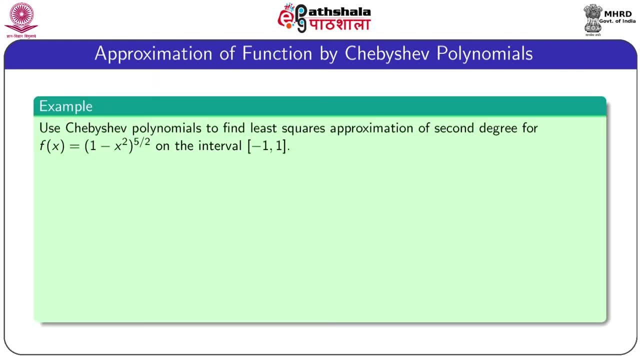 0.. So these are the orthogonality property of the Sivashvili polynomial, along with two equal cases. Now we consider one example: to approximate a function f, x equal to 1 minus x square power 5 by 2, using least square method with the: 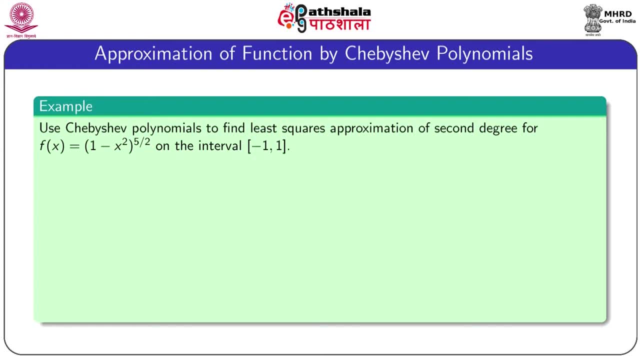 help of Sivashvili polynomial on the interval minus 1, 1.. Let the function f x is approximated at the interval minus 1, 1.. Let the function f x is approximated at the interval minus 1, 1.. 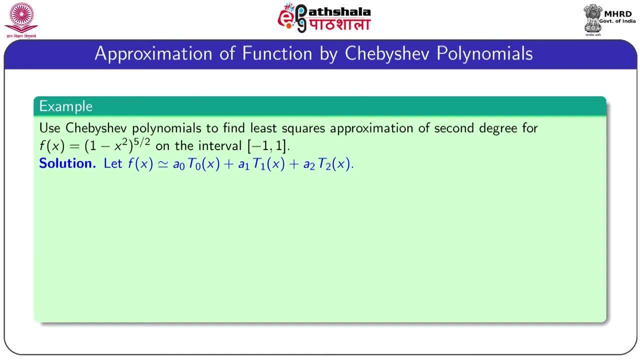 Afterride implementation started as a0- t 0 x plus a1, t 1 x plus a2- t 2 x, where t 0 x, t 1 x and t 2 x are first three Sivashvili polynomials, and a0, a1, a2 are the constant. 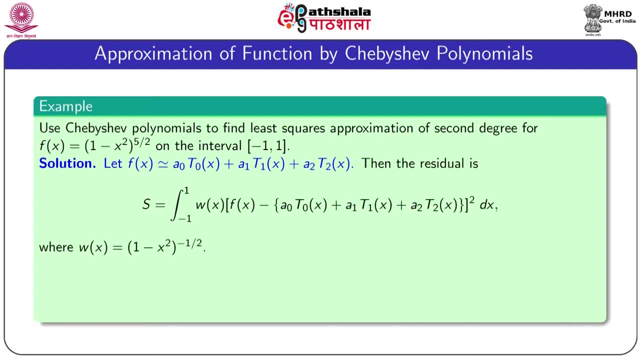 Then the residual is, as by definition of least squares method s, equal to many first years. integration minus 1 to one: w x whole into f x minus a0, into t 0 x plus a1, t 1 x, a 2, t 2 x whole to the power 2 d x, where the weight function w x equal to 1 minus x. 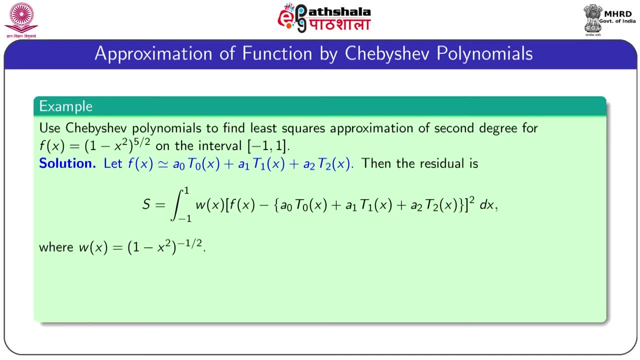 square to the power. minus of this is the weight function for Siebensche polynomial For minimum a's. we have to differentiate a's with respect to a 0, a 1 and a 2. That means del H del a 0 equal to 0, del H del a 1 equal to 0 and del H del a 2 equal to. 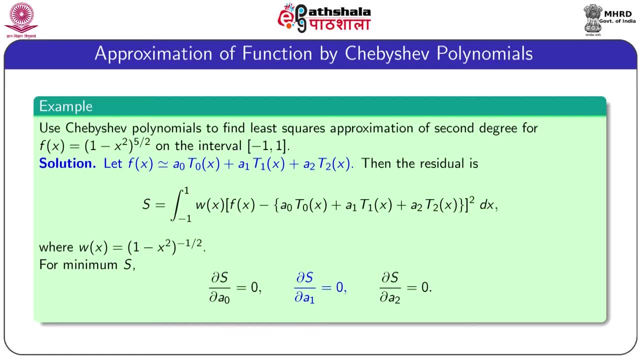 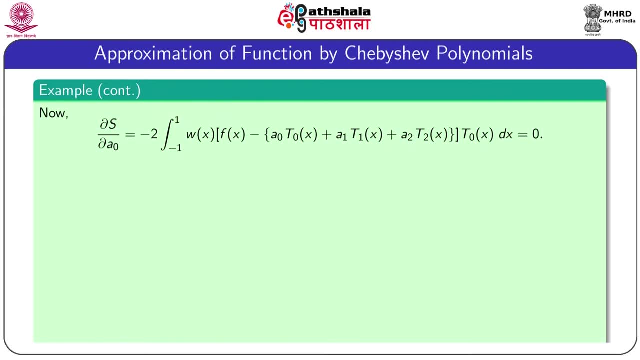 0.. So these are the normal equations to minimize a's or to find the values of a 0, a 1 and a 2.. Now, from the first equation del H, del a 0 equal to, we have minus 2, minus 1 integration. 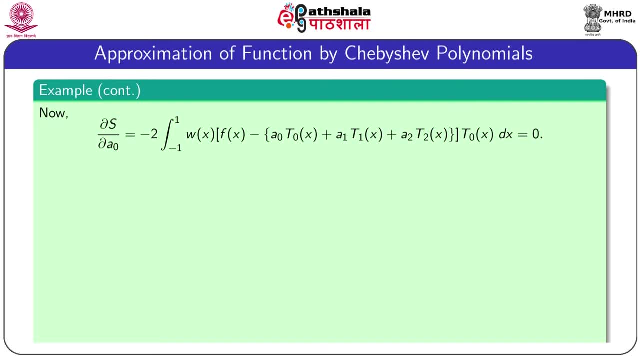 minus 1 to 1 w x into f x. minus a 0 t 0 x plus a 1 t 1 x plus a 2 t 2 x whole into t 0 x dx, which is equal to 0.. 1. 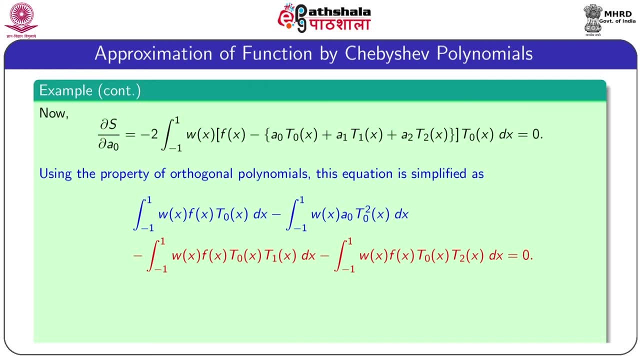 And using the property of orthogonal polynomial or after simplification this equation, the first term becomes integration minus 1 to 1 w f, t, 0, x, dx and second term is integration minus 1 to 1 w a, 0, t, 0 x power. 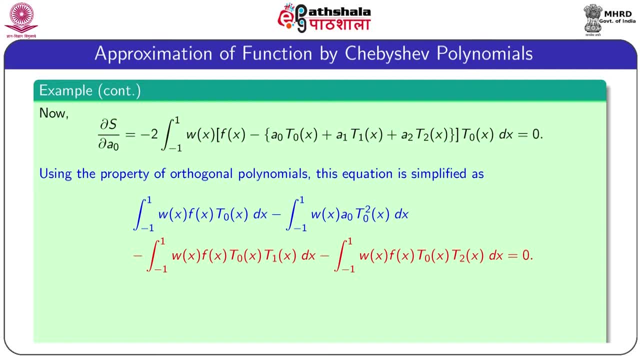 2 dx. Third term is integration minus 1 to 1 w f, t 0 x, t 1 x dx. and last term is integration minus 1 to 1 w x f x, t 0 x into t 2 x dx equal to 0.. But the last two terms are 0 because 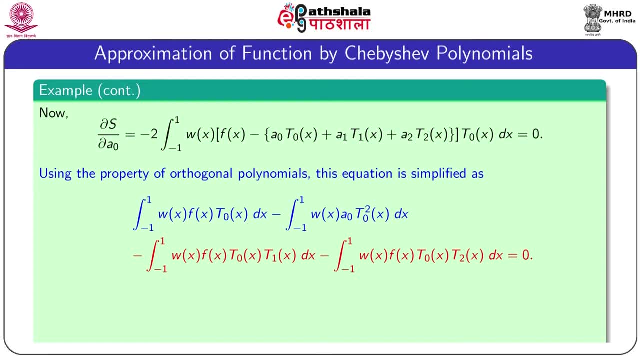 t 0 and t 1 are orthogonal. also the t 0 and t 2 are orthogonal. That is why the rate part will be discarded from this equation and we have a 0 equal to that means. from the remaining equation we can find the value of a 0, as the numerator is integration minus 1 to 1 w f. 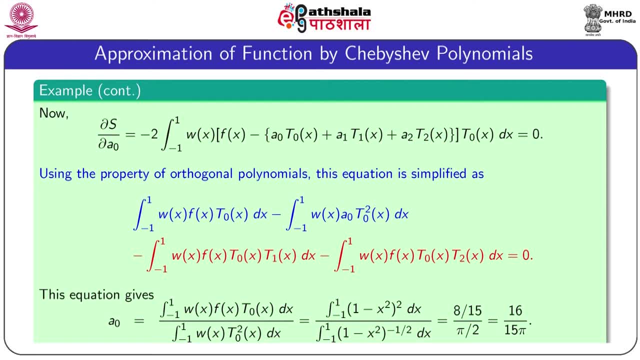 w f t 0 x dx. and denominator is integration minus 1 to 1. w f t 0 x power 2 dx. After integration, the numerator becomes 8 by 15 and denominator becomes pi by 2, and which is equal to 16 by. 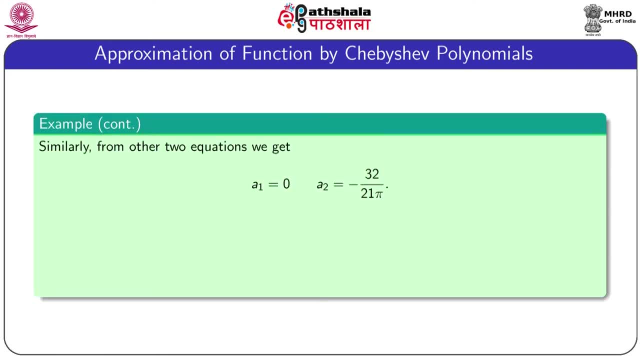 15 pi. Similarly, from other two equations we get a 1 equal to 0 and a 2 equal to minus 32 by 21 pi. So using these values, the CBC approximation of the function f x is f x equal to 16 by 15 pi into t 0 x minus. 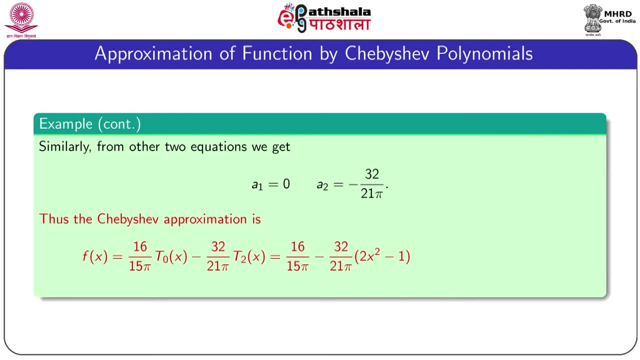 32 by 21 pi into t 2 x and after simplification this becomes 16 by 15 pi minus 32 by 21 pi into 2 x square minus 1.. 2 x square minus 1 is the value of t 2 x and after final simplification: 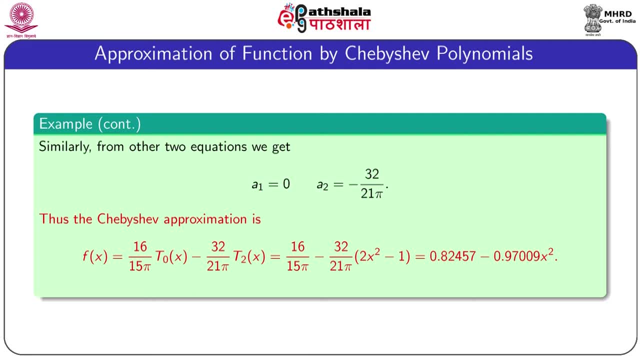 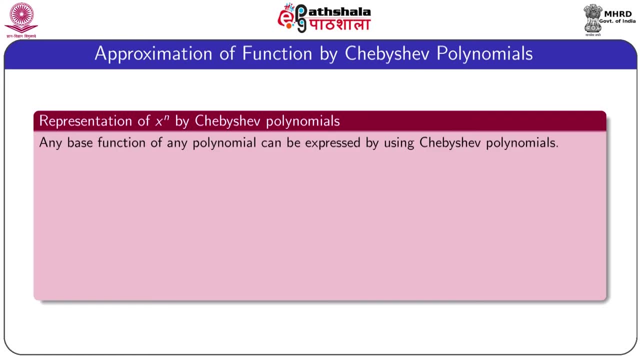 f, x becomes 0.81.. to 457 minus 0.97009 into x square. Now we can show that any power of x can be expressed in terms of symmetry polynomials. For example, one can be expressed as a zeroth order symmetry. 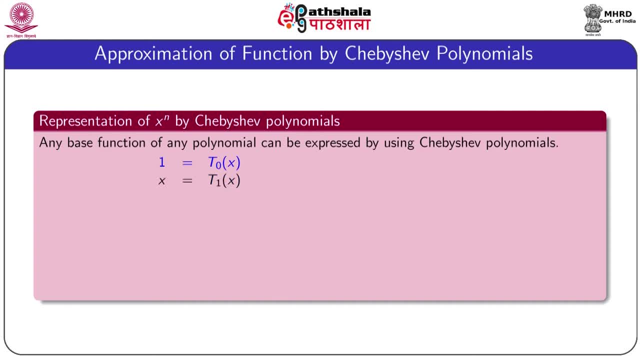 polynomial that means 1 equal to T0 x x equal to T1 x x. square equal to half of T0 x plus T2 x x. cube equal to 1 by 4, 3 into T1 x plus T3 x. Similarly, x to the power 4 can. 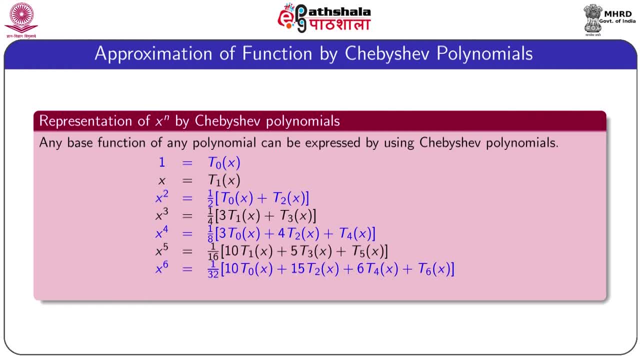 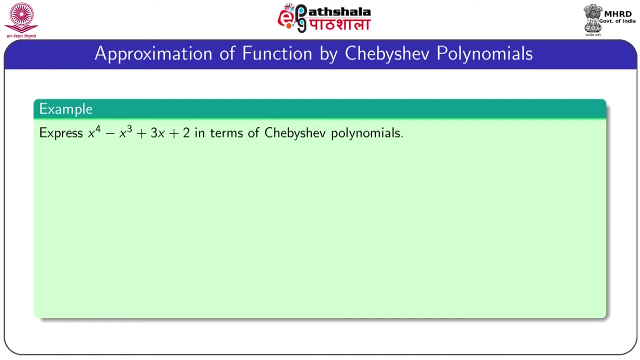 be expressed with the help of symmetry polynomials: x to the power 5 is this one. The expression for x to the power 6 is this one. and x to the power 7 is this expression containing four terms. So, using this representation, we can conclude that every polynomial can. 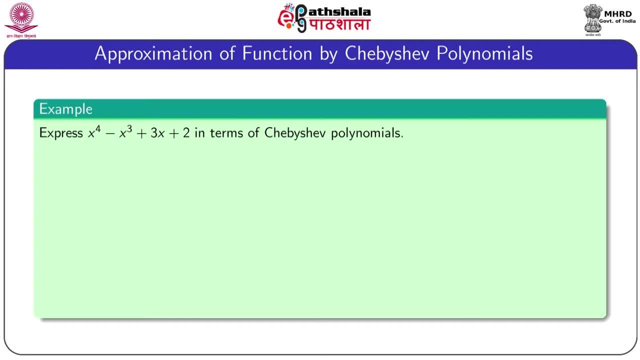 be expressed in terms of symmetry polynomial. To illustrate this concept, we considered an example. The example is express: x to the power, 4 minus x, cube plus 3, x plus 2. in terms of symmetry polynomials, We have shown that 1 equal to T0 x, that means 2 can be written as 2 into T0 x. x is nothing but T1 x and. 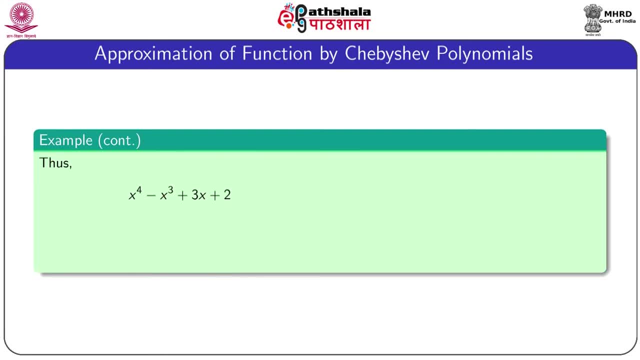 so on. So, substituting these values, the given polynomial becomes T0 x plus T2 x plus T3 x. So, substituting these values, the given polynomial becomes 1 by 8 into 3, into T0 x plus 4, into T2 x plus T4 x. This is the value of x to the power. 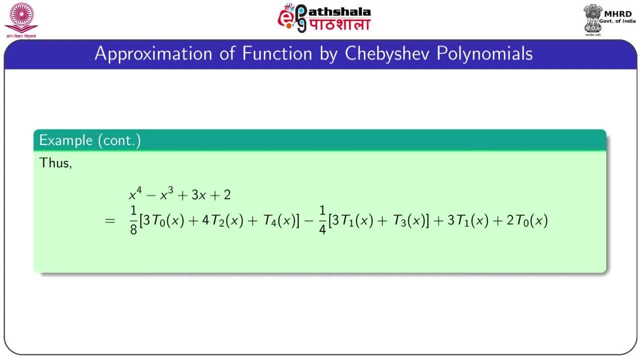 4 minus 1 by 4 into T1 into 3 plus T3 x. This is the value of x cube. And third term is 3 into T1 x and last term is 2 into T0 x. T0 x is 1.. That is why last term is 2 into. 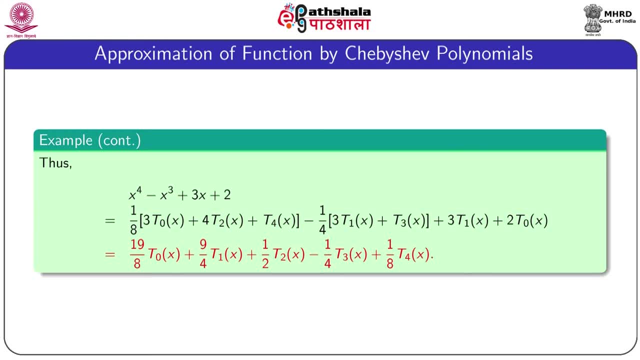 T0 x. After simplification, the polynomial finally reduces to 9.. 19 by 8 into T0 x plus 9 by 4 into T1 x, plus half into T2 x, minus 1 by 4 into T3 x plus. 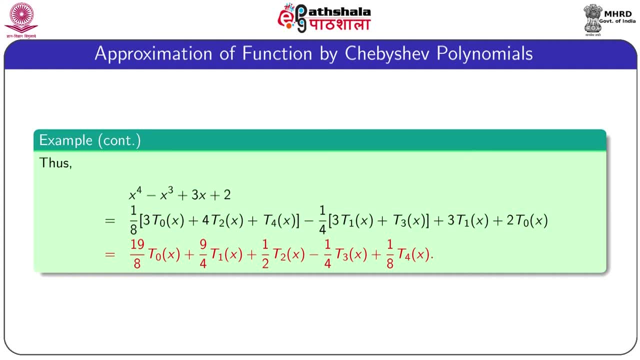 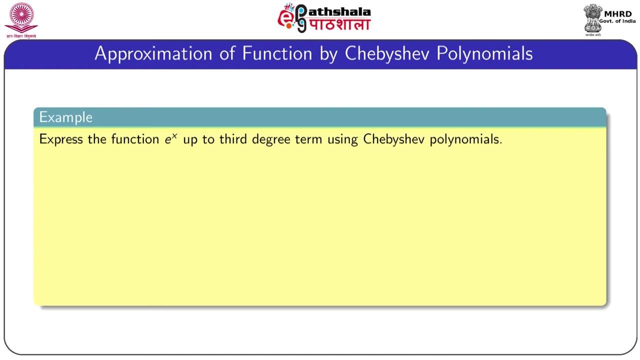 1 by 8 into T4 x. That means the ordinary polynomial can be expressed with the help of symmetry polynomials, and the degree of the symmetry polynomials is also 4.. Now we consider another example. Here we expand the function e to the power x up to third day. 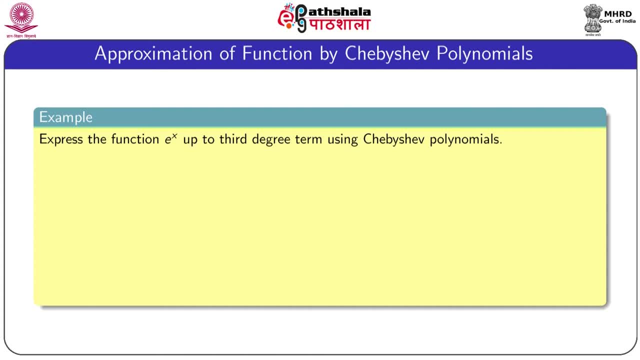 degree term. using symmetry polynomials By Taylor series expansion, we know that e to the power, x is approximately equal to 1 plus x plus x square by factorial 2 plus x cube by factorial 3.. And this expression is taken up to third degree term. Now e to the power. 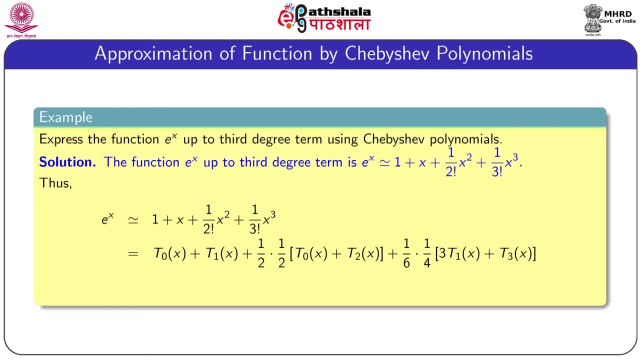 x can be expressed in terms of symmetry polynomial, because 1 can be written as 3 into T0 x, plus 1 by 4 into T1 x, plus 1 by 4 into T3 x. After simplification, this expression reduces to: 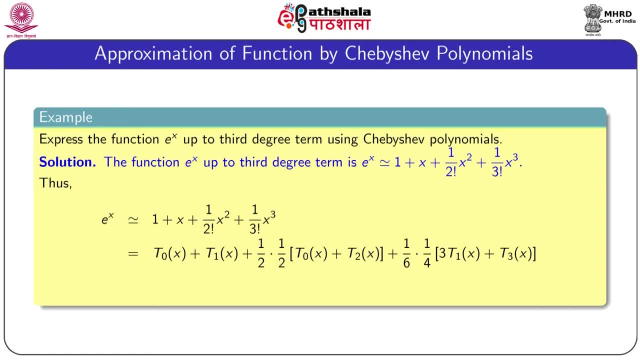 1 by 24 into 30 T0 x plus 27 T1 x plus 5 into T3 x plus 3. after simplification this expression reduces to 1 by 24 into 30 T0 x plus 27 T1 x plus 5 into T3 x plus 1 by 4, and so on. 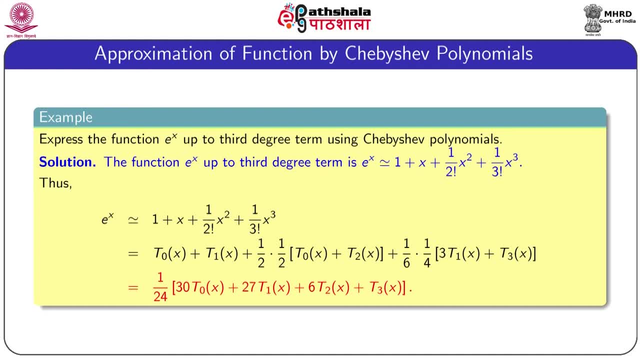 This is how we do it. Let me show you another example. Let me show you a simple example of a simple equation: plus 6 into T2x plus T3x. So the Taylor series approximation contains third degree terms. up to the third degree terms and after approximation with the help of specific polynomials, the 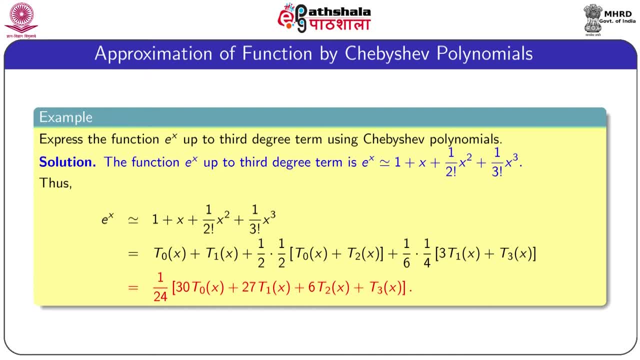 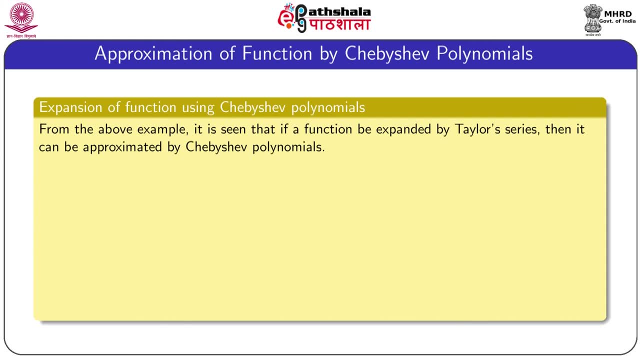 final expression is also a polynomial of degree 3.. Now we consider another kind of problem. From this example we see that if a function be expanded by Taylor series method, then it can be approximated by CBC polynomials. So for this purpose we assume that y, equal to fx be a function and which is to be approximated. 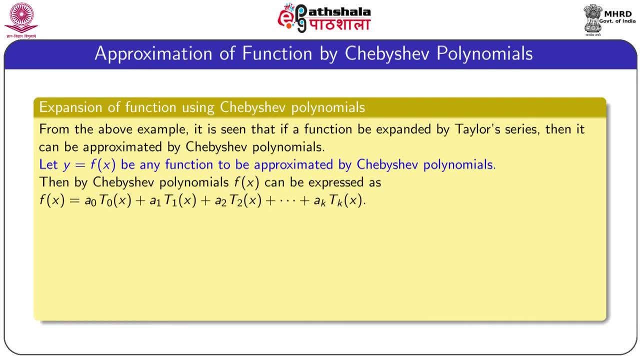 by CBC polynomials, Let the function fx be expressed as: y equal to fx, plus y equal to a0, T0x plus a1, T1x plus a2, T2x and dot, dot, dot plus ak, Tkx. where a0, a1, a2 up to ak. 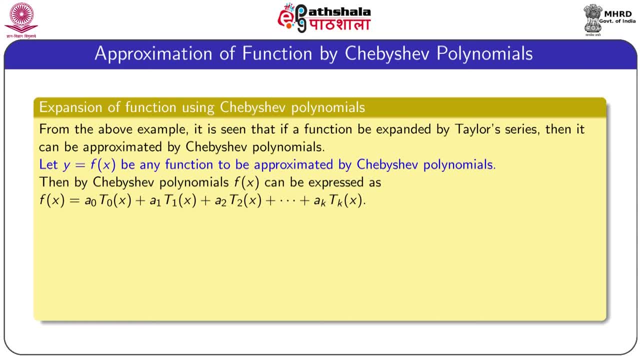 are the constant and T0x, T1x up to Tkx are the CBC polynomials of different order And the coefficient ai- that means the constant ai are given by ai equal to the numerator- is the integration minus 1 to 1, y t i a1, y t i a2, y t i a2, y t i a1, y t i a2, y t. 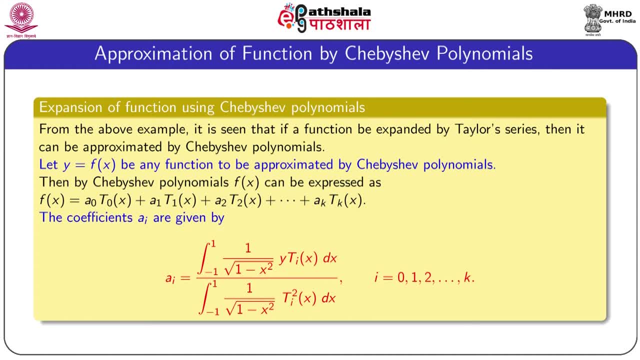 i x divided by 1 minus x square dx, and denominator is integration minus 1 to 1. T i square x whole divided by 1 minus x square dx, And this is true for i equal to 0,, 1,, 2 up to k. So using: 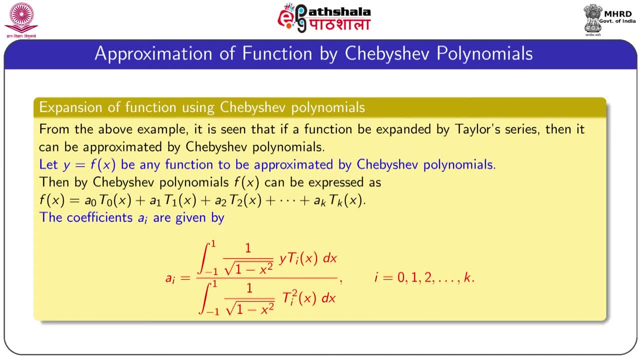 this formula we can determine the values of a0, a1 up to ak. So after computation of ai for a given function y, we can approximate the function fx with the help of CBC polynomials. So, after computation of ai for a given function y, we can approximate the function fx with: 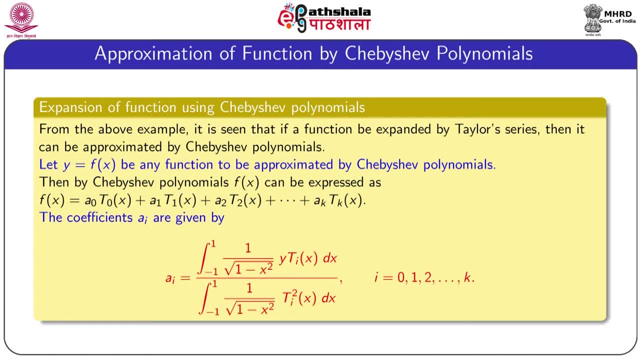 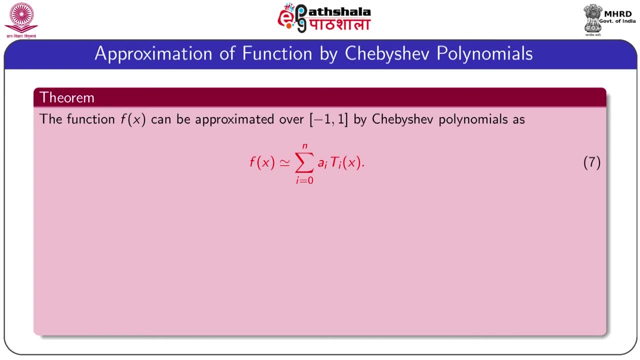 the help of CBC polynomials. Now we consider a theorem which gives the condition for which a function in a arbitrary function can be expanded or approximated over the interval minus 1, 1 by CBC polynomial. For this purpose we assume that fx is approximately equal to summation over i equal to 0 to n. 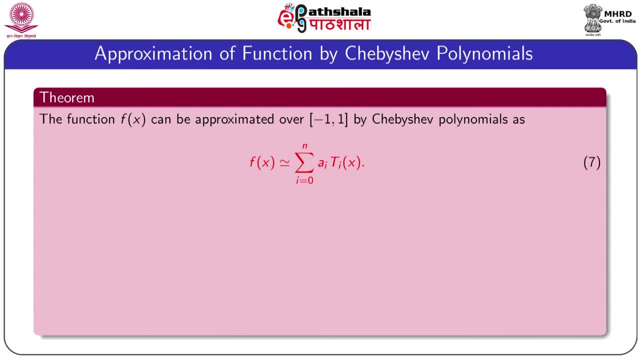 ai, T i, x, where ai is a constant obtained by the formula given in previous slide And T? i are the CBC polynomials where the coefficient a i's are given by this formula: restaurants. The first constant, a, 0, is equal to 1 by n plus 1 into summation j, equal to 0 to n- f. 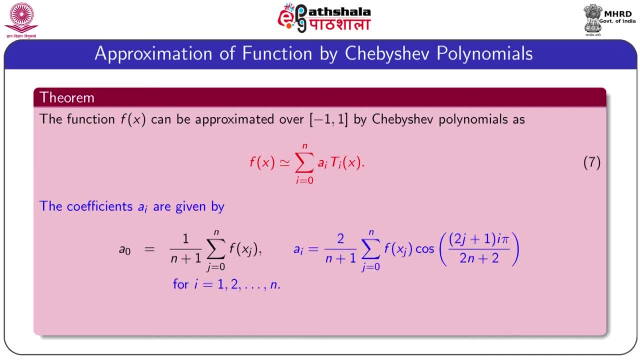 of xj and ai, equal to 2, by n plus 1 into summation j equal to 0 to n, f of x, j into cos of 2j plus 1, whole into i pi divided by 2n plus 1.. And therefore this is actually a róture and angle can be obtained by Device Rahmen. 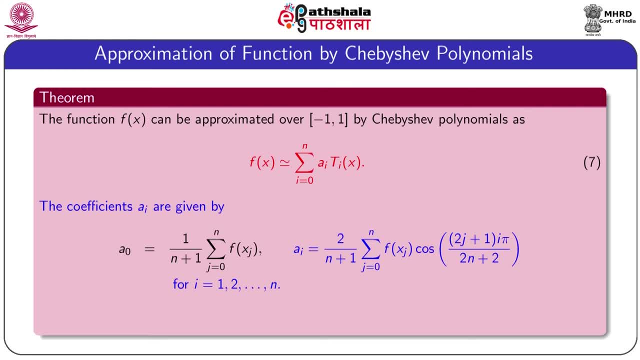 butensions and Photo配 лай크. 0, 0,T, i are the CBC polynomials. Amy Huerstein. Angular ік 0,0,N. interrogart enough, Where the coefficient a i is is given by this formula: the first constant a 0 is equal to 1 by n plus to xj into cos 2j. 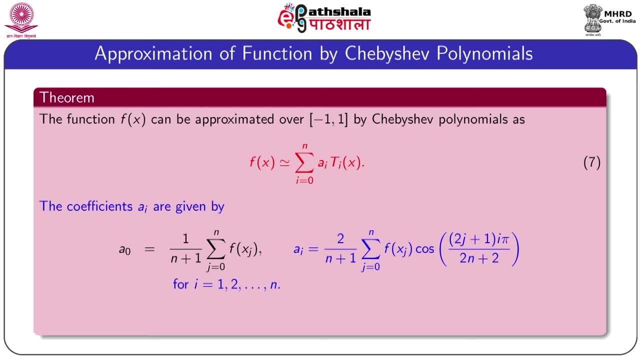 2n plus 1.. And this is true for all i equal to 1 to n. Also, the argument xj equal to cos of 2j plus 1 into pi whole divided by 2n plus 2.. So this is the expression, or this: 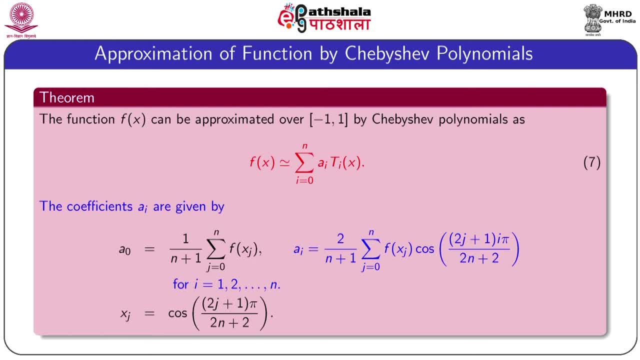 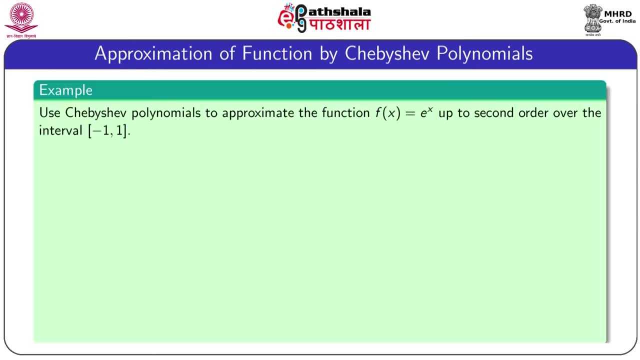 is the formula to calculate a is x. and finally, the function fx. Now here we consider a function fx equal to e, to the power x, and we have to approximate this function up to second order over the interval minus 1, 1.. The second order: citizenship. 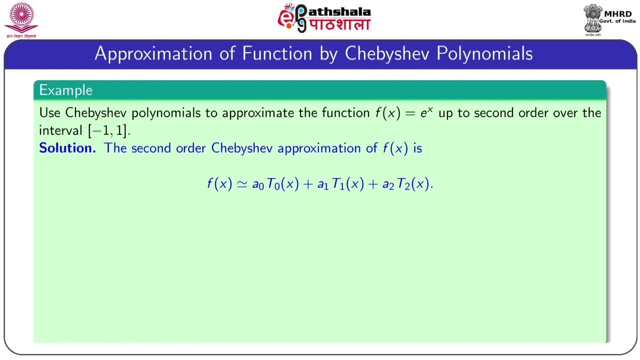 approximation of fx. is fx equal to a 0, t 0 x plus a 1, t 1 x plus a 2, t 2 x where a 1, t 1 x plus a 2, t 2 x where a 1, t 1 x plus a 2, t 2 x where a 2, t 2 x where a. 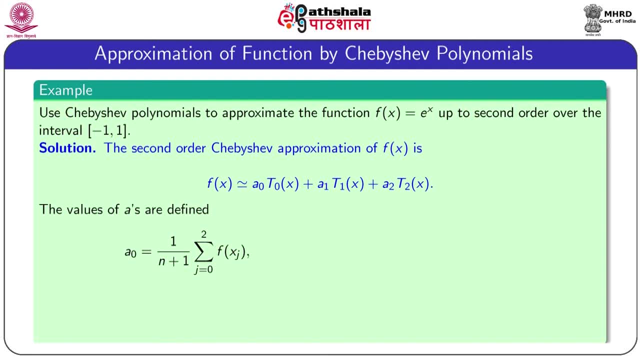 0 equal to 1 by n plus 1 into summation over j equal to 0 to 2. f of xj and a 1 and a 2 are given by this formula And the value of xj are given by xj equal to cos of 2j plus. 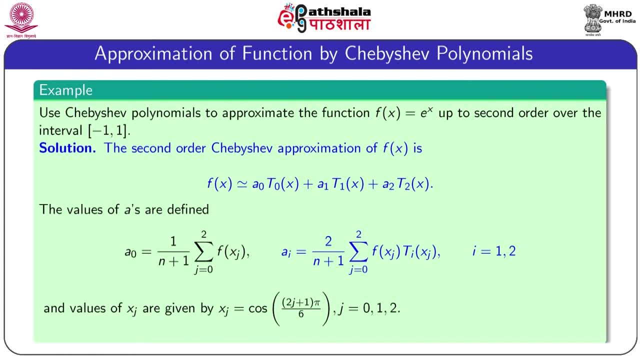 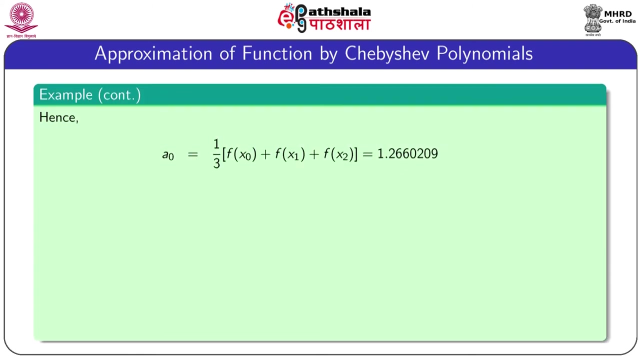 1 by 6, where j equal to 0,, 1 and 2.. That is x0 equal to 0.86660254, x0 equal to 0.86660254, x1 is 0 and x2 equal to minus 0.86660254.. Therefore, a0 equal to one-third of f of. 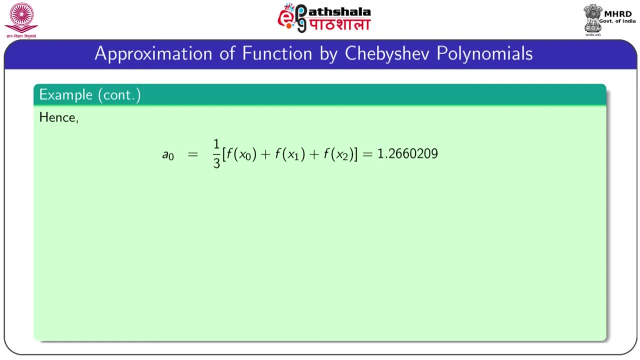 x0 plus f of x1 plus f of x2, which is equal to 1.2660209, after substituting the values of f of x0,, f of x1 and f of x2.. a1 is equal to 1.129721 and a1 is equal to 1.129721.. So. 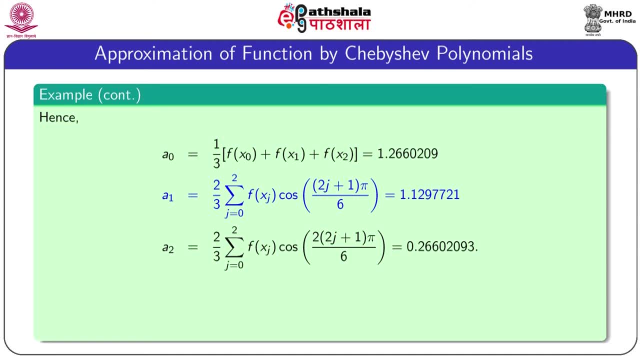 this is the offices of the formula with x and in both cases We know that f is計ing a, 0,d crayon, x, t or c. Of course, we know that f of x is equal to a value of x limitations, xj, a2 equal to 0.2660209, and a2 is equal to 0.266020・ Про. 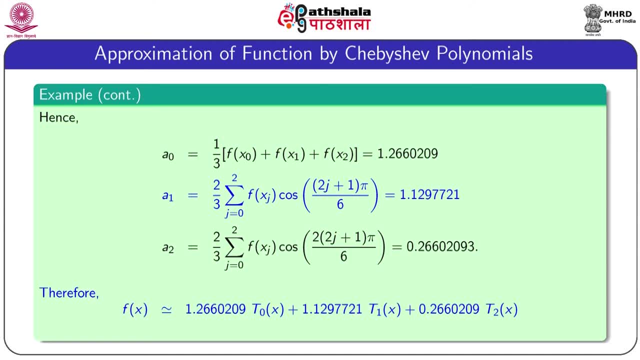 x. Therefore, the function fx is approximately equal to 1.2660209 into t0 x plus 1.129721 into t1x, plus 0.2660209 into t2 x And after substituting the values of t0ят Xavierkeaș. 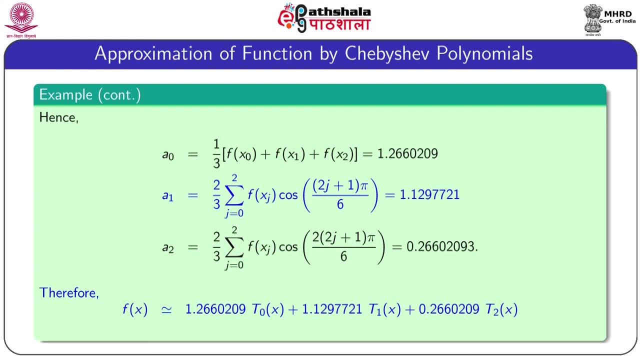 x, T1 x and T2 x. this expression becomes 1 plus 1.129721, x plus 0.5320418 into x square. So this is the approximate value of e to the power x within the interval minus 1, 1 and this expression. 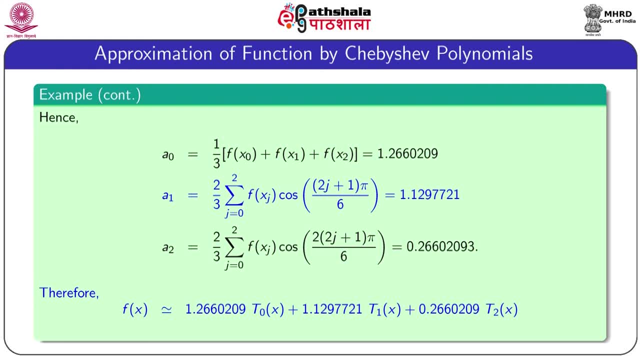 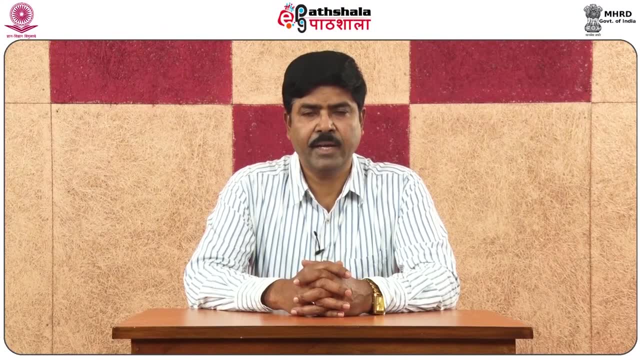 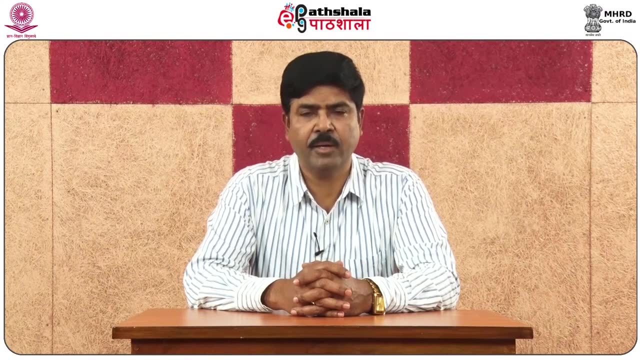 is taken as the up to the quadratic terms, that means the second degree terms. So we have defined Sibeshi polynomial Tn, x and have shown that a Sibeshi polynomial is even function or odd function, according as the degree of the polynomial is even or odd. 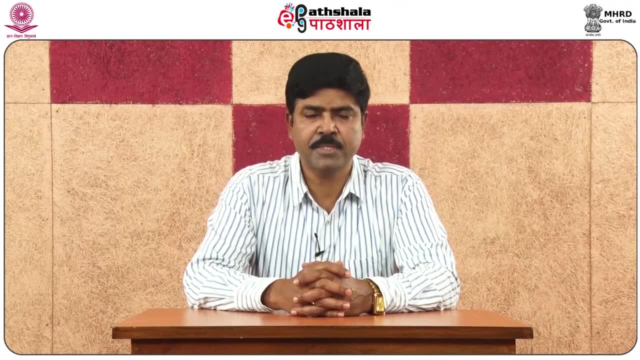 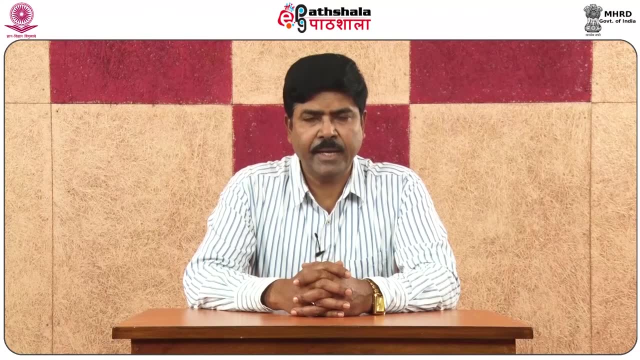 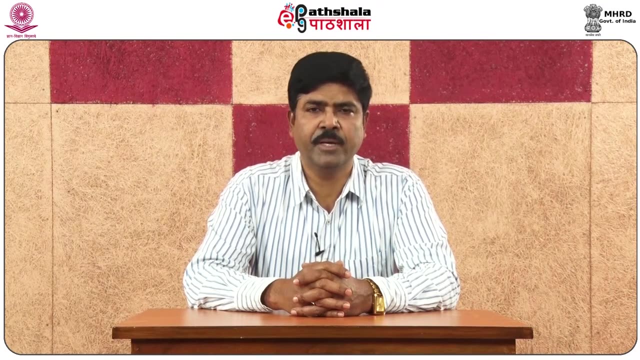 Also, we have shown that all the Sibeshi polynomials can be deduced or generated from a recurrence relation. Also, it is highlighted that the every function can be expanded with the help of Sibeshi polynomial, provided the function has a valid Taylor series expansion. 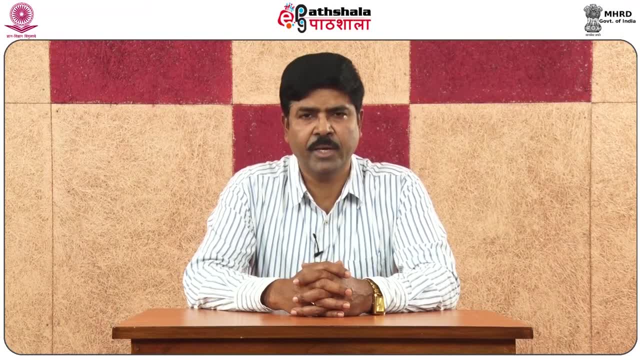 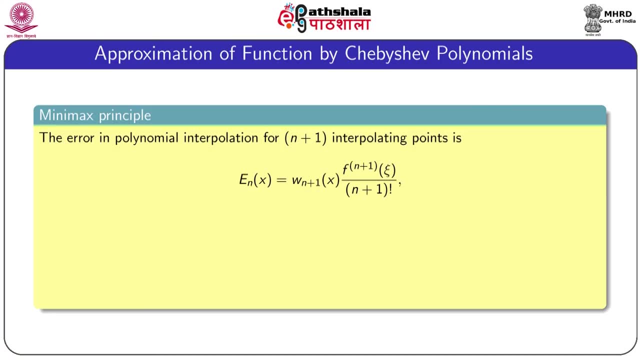 Now we define the minimax polynomial and we shall state the minimax principle which is used to optimize the error. In chapter 2, we have shown that the error in polynomial interpolation for n plus 1 interpolating points is e, n, x equal to w, n plus. 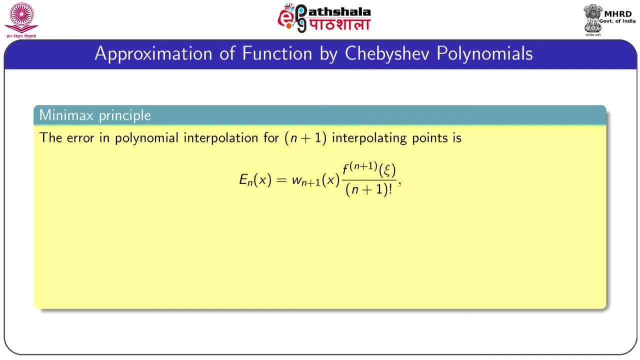 1 of x into n plus 1. derivative of the function f at the point xi, divided by factorial n plus 1, where w n plus 1 of x is a polynomial of degree, n plus 1, which is equal to x minus x. 0 into x minus. 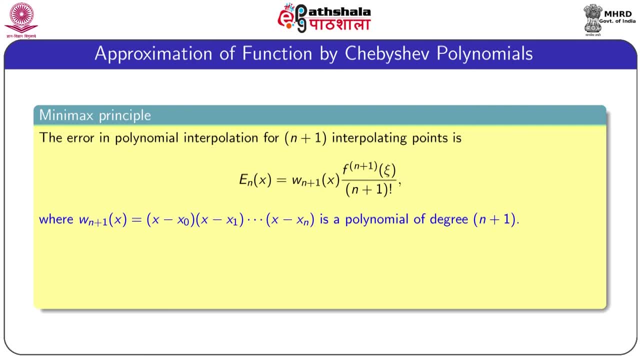 x 1 up to x minus x n. Now it is obvious that the upper bound of the error can be determined by the following expression. that means the absolute value of the error- e n, x- is less than or equal to maximum over the interval minus 1, 1 of absolute value of w n, plus 1 of x into the maximum value. 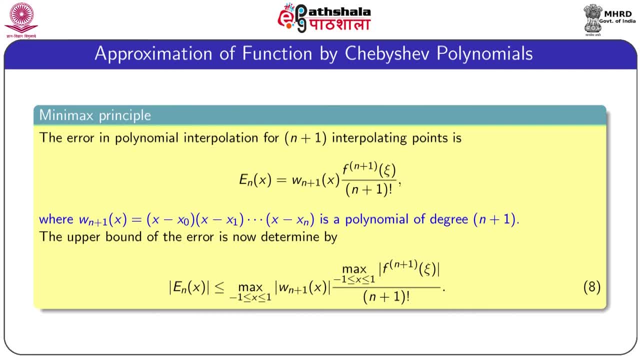 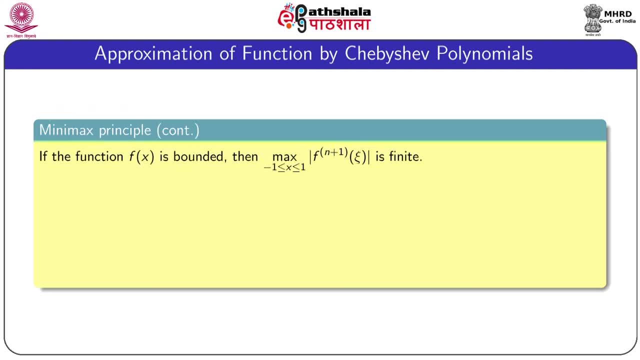 over the interval minus 1, 1 of n plus 1 derivative of f at xi by factorial n plus 1.. If the function f, x is bounded- that means the given function is bounded- then obviously the maximum value of the n plus 1 derivative of f at any arbitrary point xi is finite. 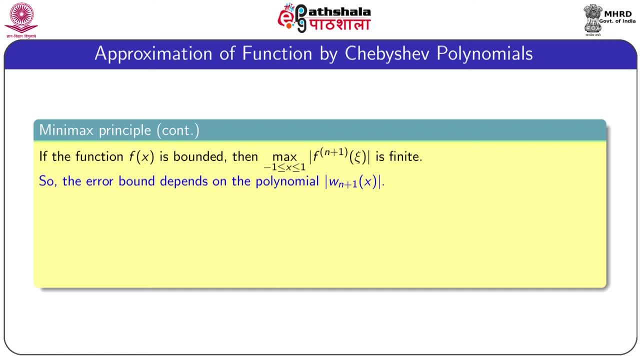 So the error bounds depends only on the polynomial Wn plus 1 of x. Again, the absolute value of the polynomial Wn plus 1 of x depends only on the choices of the nodes or arguments x0, x1 up to xn. Thus the maximum error depends on the product of two terms. 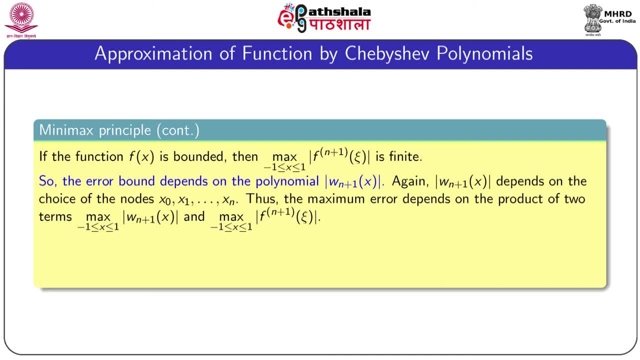 one is the maximum absolute value of Wn plus 1 of x, and other is maximum values of the n plus 1 derivative of f at xi. But the CBSChip suggested that the arguments x0 to xn must be chosen in such a way that the argument to be chosen is of absolute value, is only x1 of C and the argument to be chosen is of absolute values of x0 and xn. The CBA-SHIP suggested that arguments x0 to xn must be chosen in such a way that 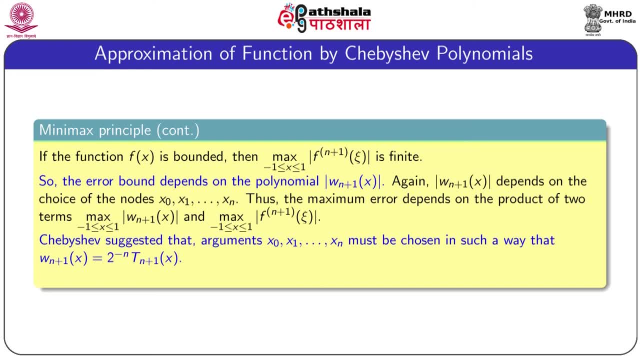 Wn plus 1 of x equal to 2, to the power minus n into Tn plus 1 of x. Note that Tn plus 1 of x is a polynomial of degree n plus 1.. Also, the polynomial Wn plus 1 of x is also a polynomial. 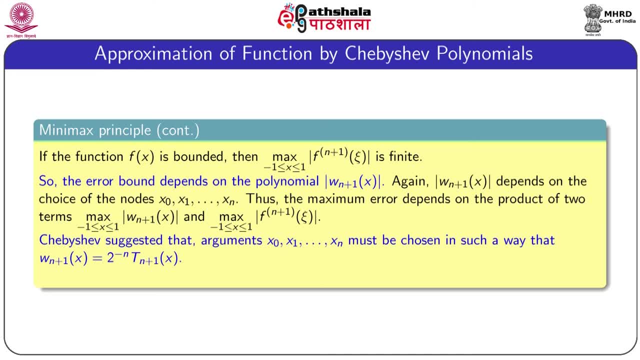 of degree n plus 1.. Also, the leading term of the polynomial Tn plus 1 is 2 to the power 1 by 2 to the power n. That is why we have considered Wn plus 1 of x equal to 2 to the. 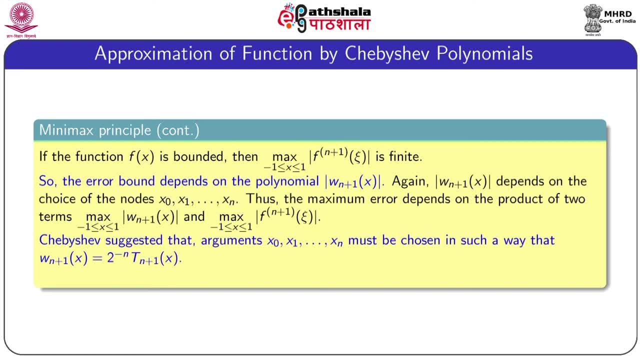 power minus n into Tn plus 1 of x. The polynomial 2 to the power minus n into Tn plus 1 x is a monic Cveschi polynomial and it is denoted by T tilde n plus 1 x. Thus the polynomial. 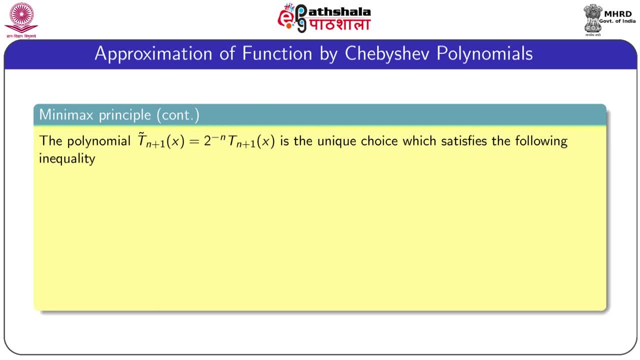 T tilde n plus 1 of x, equal to 2 to the power, 1 by 2 to the power n. The polynomial T tilde n plus 1 of x, equal to 2 to the power minus n, into Tn plus 1 of. 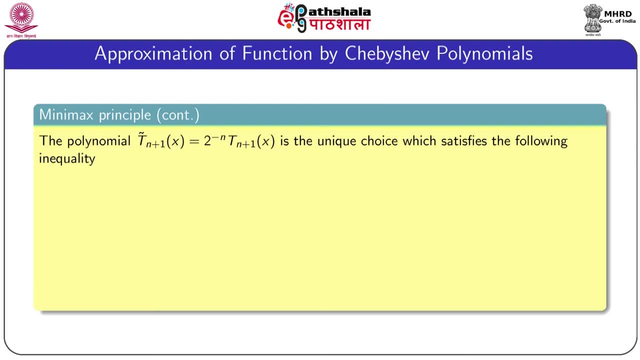 x is the unique choice which satisfies the following inequalities. That means the maximum value of the T tilde, n plus 1 of x over the interval minus 1, 1 is less than or equal to the maximum value of Wn plus 1 of x over the interval minus 1, 1.. Again, the absolute. 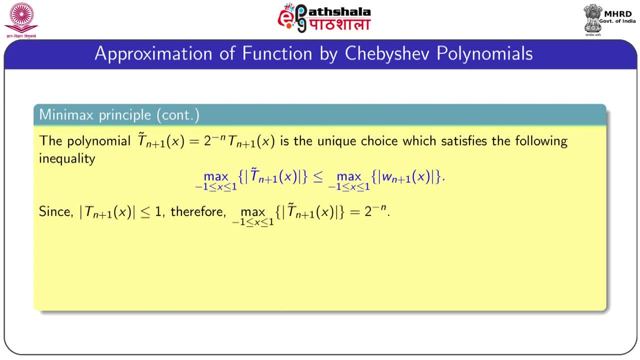 value, or the maximum value of Tn plus 1 of x, is 1.. Therefore, the maximum value of T tilde n plus 1 of x, that means the absolute of the maximum values of this function over the interval minus 1, 1, is equal to 2 to the power. 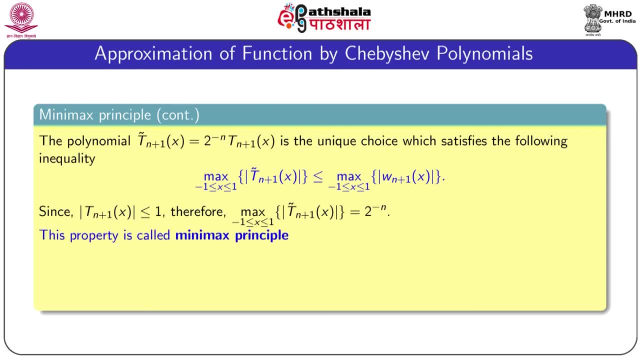 minus n. This property is called the minimax principle and the polynomial T tilde n plus 1 x equal to 2 to the power minus n, into Tn plus 1 x or T tilde n of x equal to 2 to the 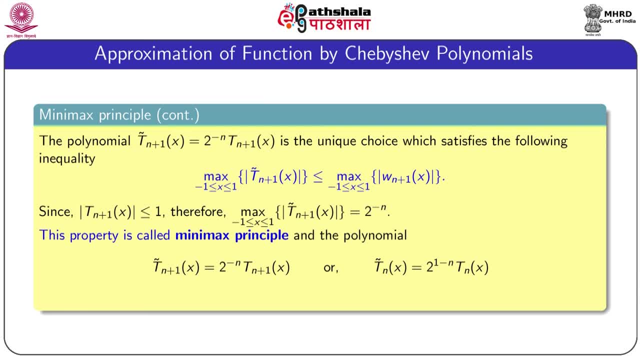 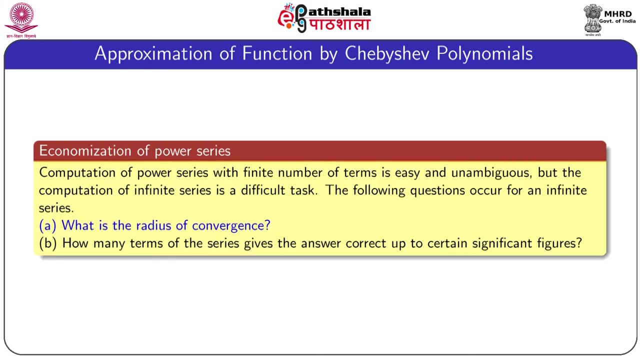 power 1 minus n into Tn of x. This polynomial is called minimax polynomial. That means, using this polynomial we show that the error in interpolation, polynomial interpolation, must be minimized. Now we describe another application of Munf-Cveschi polynomials In economization of power series. 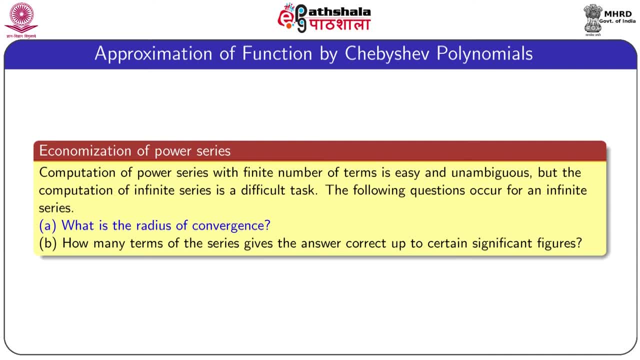 we have seen that components e to the power n and e to the power t are the common움. We have seen that computation of power series with finite number of terms is very easy and unambiguous, but the computation of infinite series is a very difficult task. 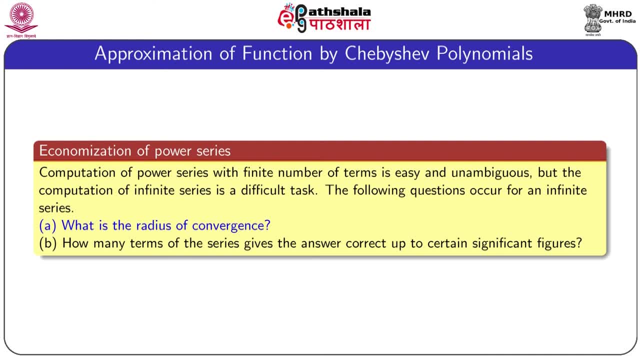 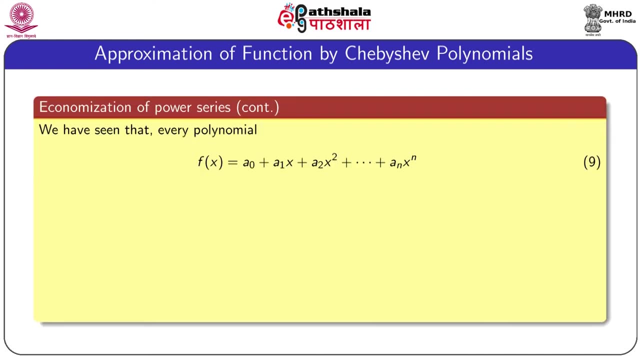 The following questions occur due to computation of an infinite series. The first question is: what is the radius of convergence, and other is how many terms of the series gives the answer correct up to certain significant figures? Now we have seen that every polynomial f of degree n can be expressed in terms of: 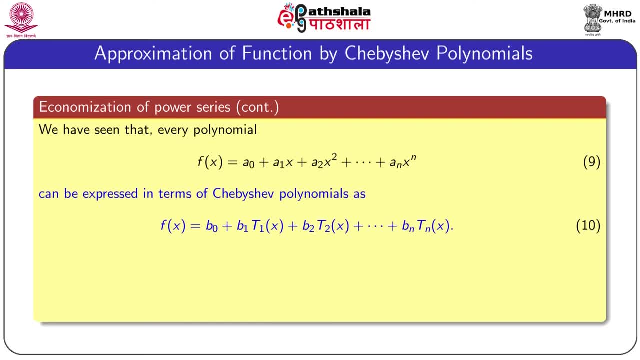 CBC polynomials as the following: form: f equal to b0 plus b1, t1 x, up to bn, tn, x. and it can be shown that the expansion of the form tan converges more rapidly than the form of equation 3.. Thus the representation of tan of any function or any polynomial f is computationally: 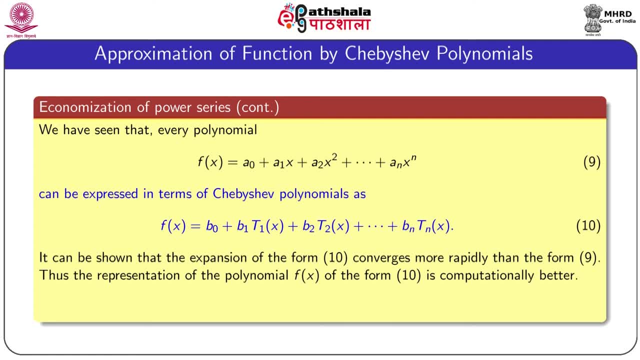 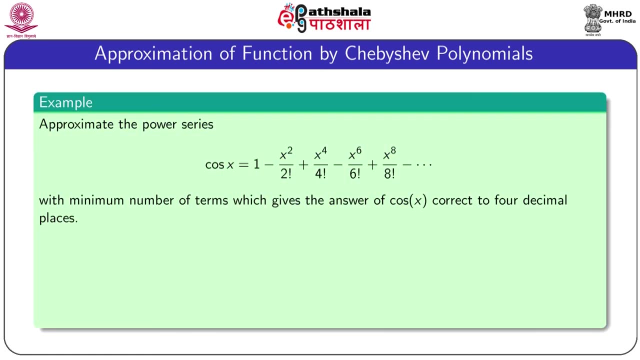 better than that of 9.. The computation of a power series with least number of terms or least amount of time, which gives the desired accuracy, is called the economization of the power series. Now we explain this method- economization of power series- With an example. here we consider the cosine series, which is nothing but 1 minus x square. 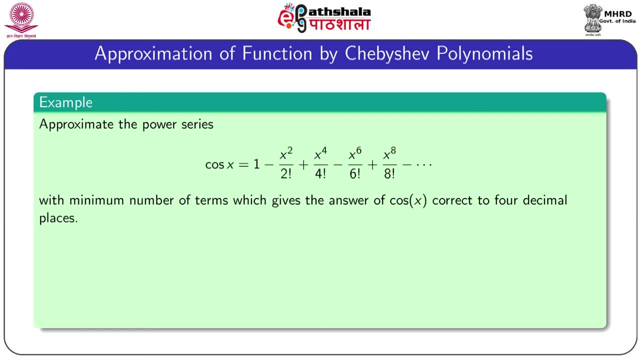 by factorial 2 plus x to the power 4, by factorial 4 minus x to the power 6, by factorial 6 plus x to the power 8, by factorial 8 minus dot dot dot. Our aim is to find the finite approximation of the series cos x, and that gives the answer. 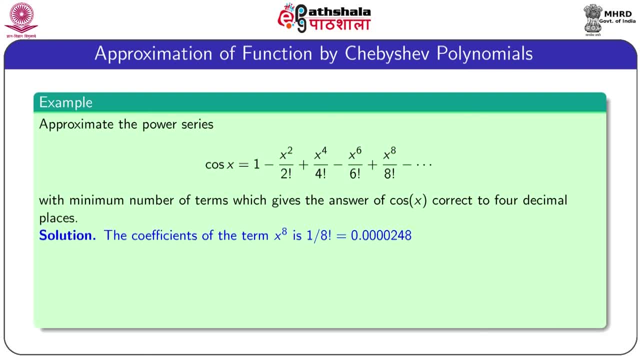 correct up to four decimal places. Thank you. Note that the coefficient of the term x to the power 8, x to the power 8 is 1 by factorial 8, which is equal to 0.0000248, and note that it is effected in the fifth decimal place. 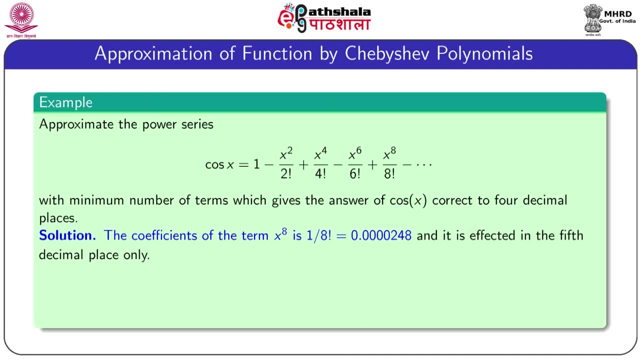 only because the first four digits are zeros. therefore there is no effect in the first four terms in the calculations. So we can. We can truncated the term x to the power 8 by factorial 8 and other higher power terms from the given series. 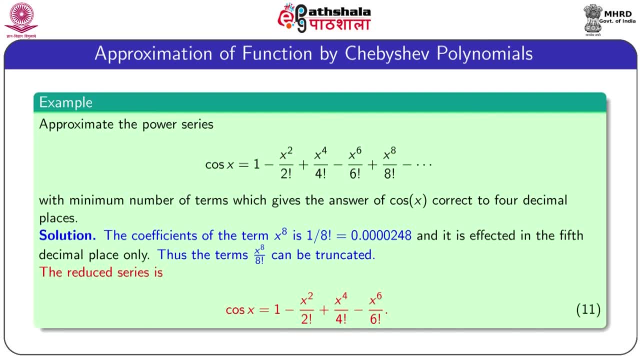 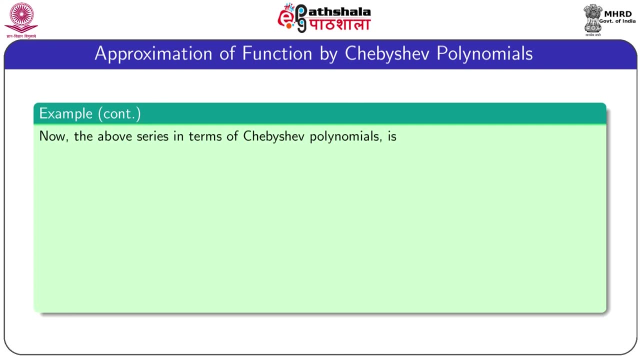 And the reduced series is cos x equal to 1 minus x square by factorial 2 plus x to the power 4 by factorial 4 minus x to the power 6 by factorial 6.. Now we use the Sibeshi polynomial to approximate this function. 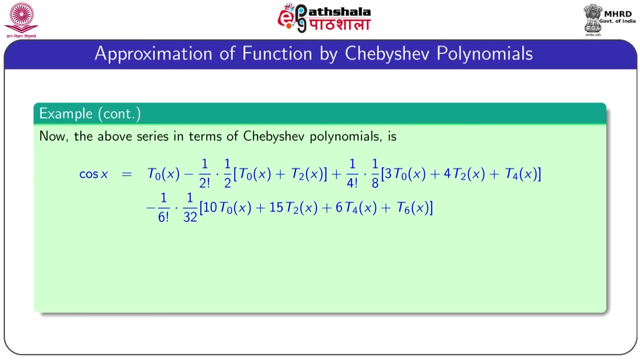 After substituting the Sibeshi polynomials, The cos x becomes this expression and after simplification, this reduces to cos x equal to 0.7651910 minus 0.2298177 into T2, x plus 0.0049479 into T4, x minus 0.0000434 into T6. 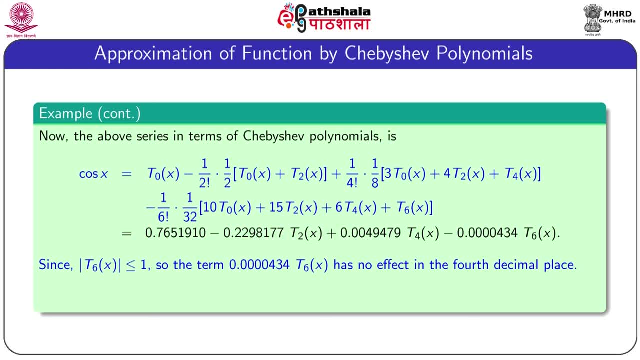 x absolute value of T6X is less than or equal to 1.. Therefore, the last term of the above expression, or the term 0.0000434 into T6X has no effect in the fifth decimal place. Therefore, the term is discarded and the reduced economized series is given by cos X equal. 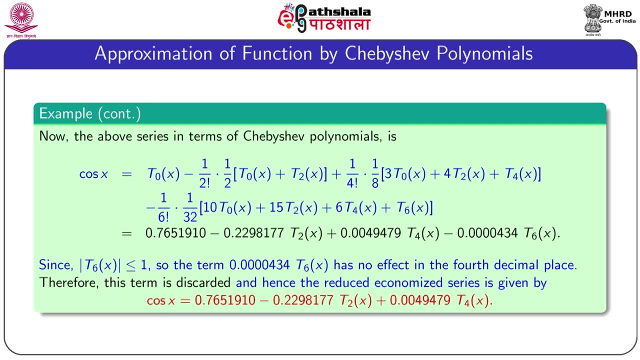 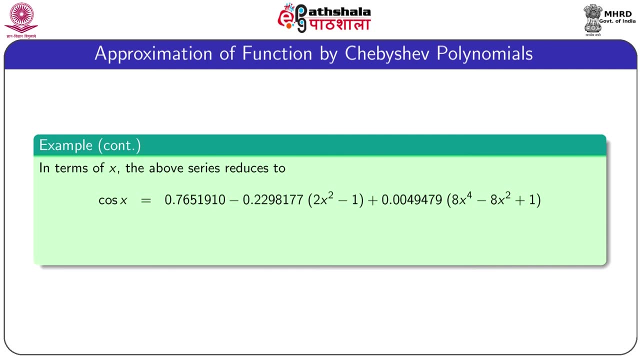 to 0.7651910 minus 0.2298177 into T2X, plus 0.0049479 into T4X, And after substitution of the values of T0, T1, T2 and T4X, we get cos X equal to 0.7651910 minus 0.2298117.